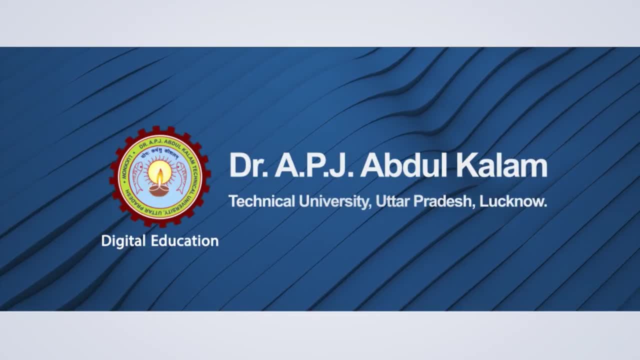 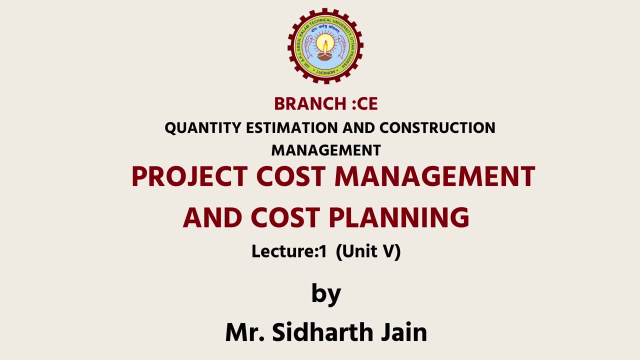 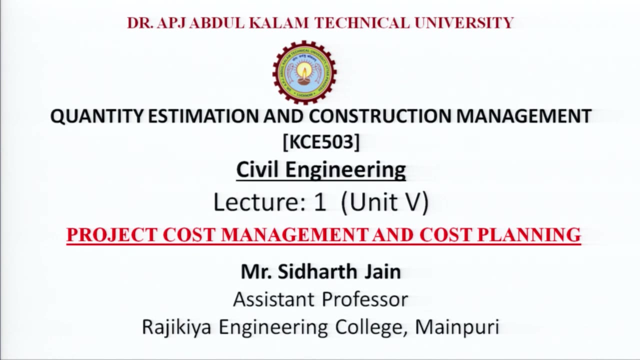 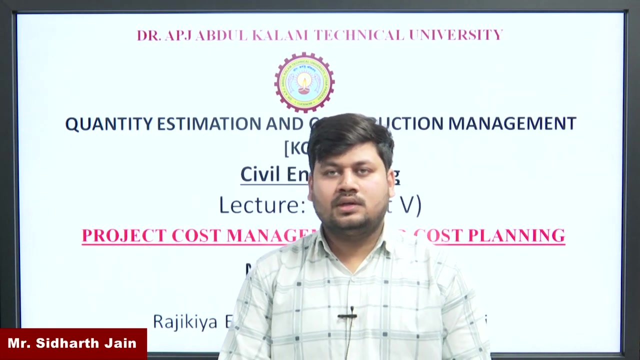 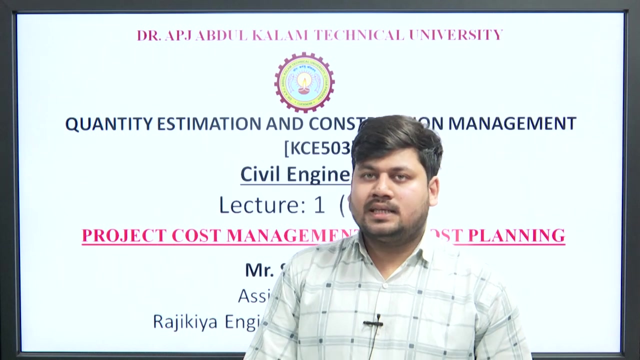 Hello students, this is Darjan, a session professor from the Rajki Engineering College, Mahanpuri. This is the first lecture of unit 5th of our subject Quantity Estimation and Construction Management. In this lecture we will understand about the project cost. 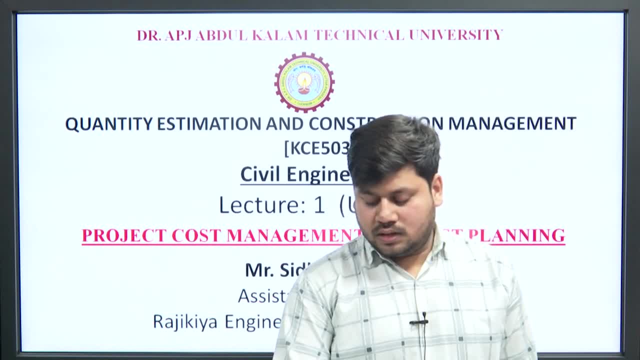 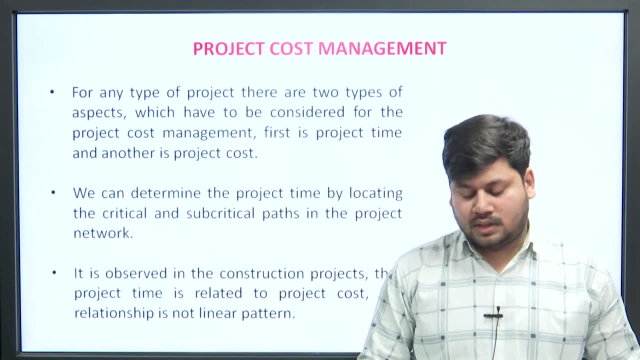 management and the cost planning. So what is project cost management? Basically, project cost management means to manage the cost of the project. we do not want the maximum cost To bring the minimum cost of the project. we call it as optimum cost To bring the optimum. 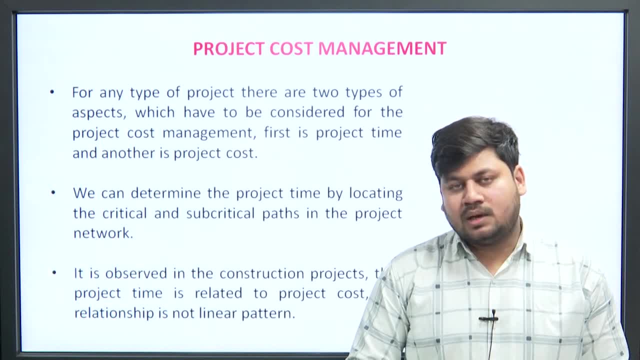 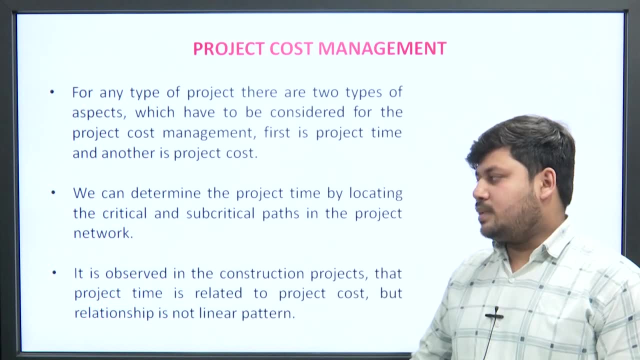 cost. we call that as project cost management, But we also have to look at the other aspect too. if we talk about the first one, for any type of project there are two types of aspects which has to be considered for the project cost management. First is a project time and 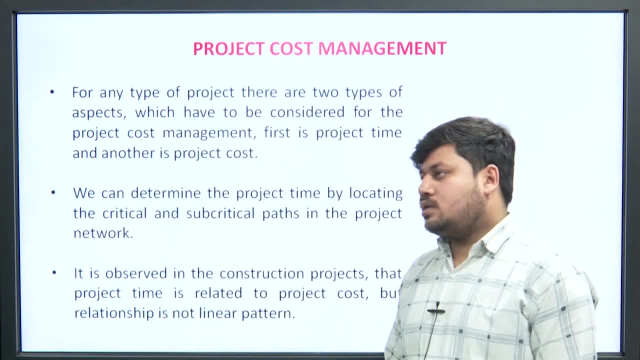 the second one is a project cost. basically, If we want to see project cost management, then we have to look at the other factor, project time, apart from the project cost. It should not happen that if we reduce the project cost, then in that case we can also see the second. 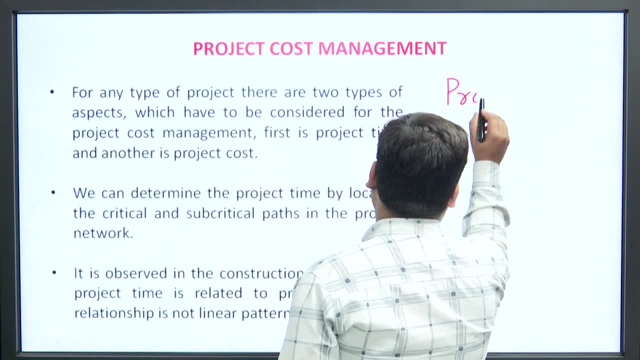 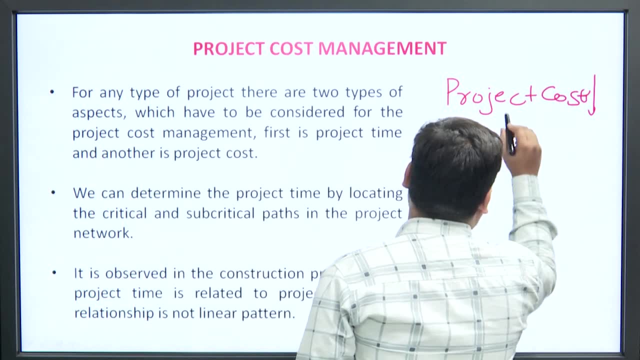 aspect: the project time. We will have to look at the project time. It should not happen that If we want to reduce the project cost, we have to reduce it. if we want to reduce the project cost, then due to that, our time is the project cost- it will go very far ahead. 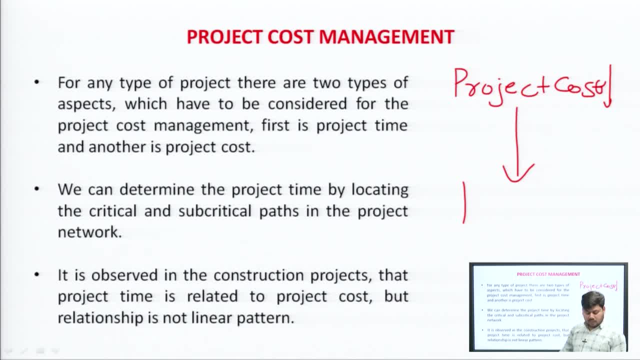 we do not want this. we will have to take the project cost and project time in the same way, So we can determine the project time by the locator. it is observed that the construction project, that project time, is related to the project cost. we understand some things, for. 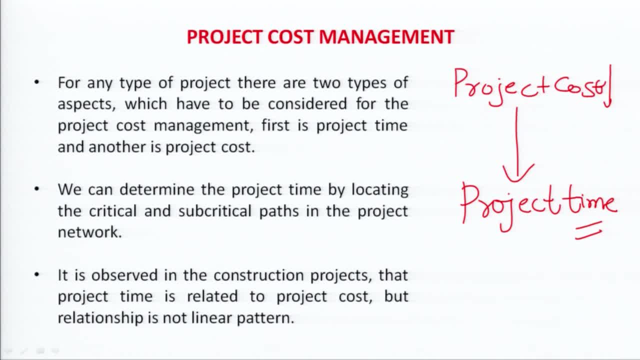 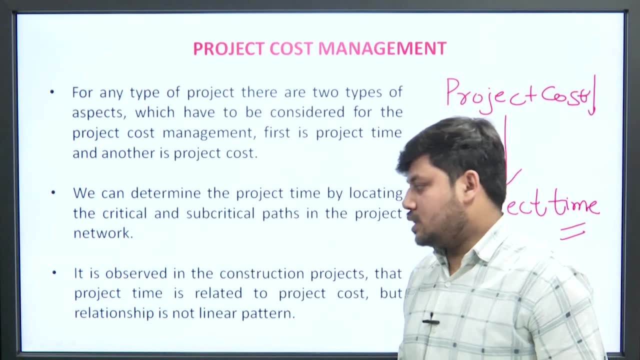 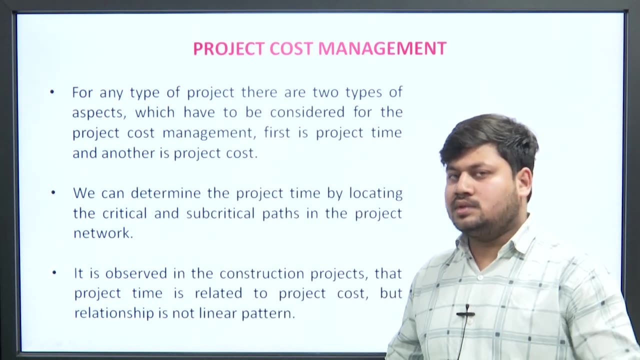 the project cost management. What is the meaning of project cost management? Let us understand this first. Project cost management means that we have to keep the cost of our project at the least. we have to try to keep it as low as possible. But we have to look at the second term or aspect of project time, along with keeping the project. 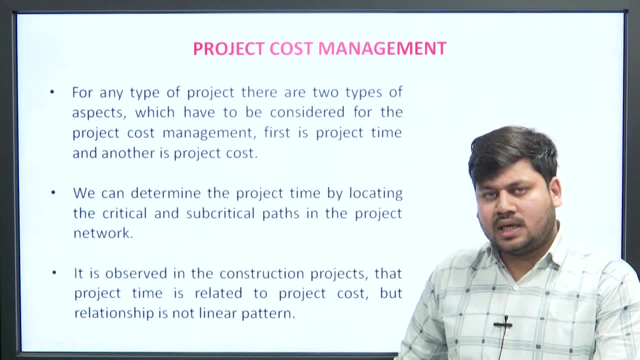 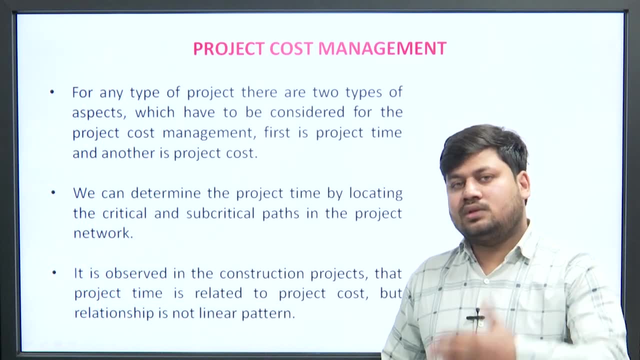 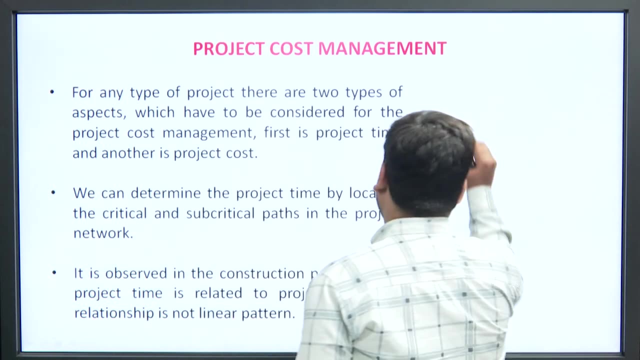 cost low, that if we are reducing the project cost, then due to this, our project time is not increasing. our limiting time is not increasing. it is not increasing for a particular time. we have to see that too. So we have to rear a even time in the project because the time of completion of a project 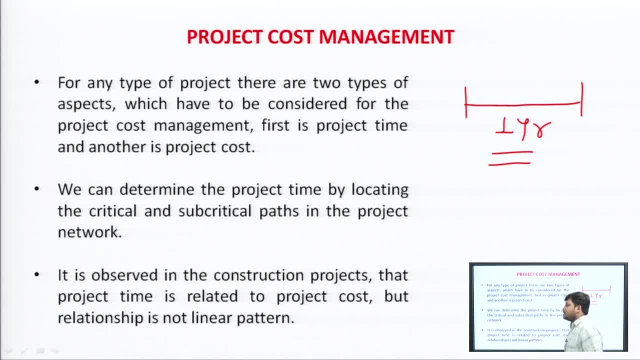 is one year, Suppose for a project, it is one year. then in one year's project completion, how can we reduce our project cost? that is called as project cost management, in the simplest way. Now, how will we reduce the project cost? We will reduce the project cost in the way that we will see the critical and subcritical 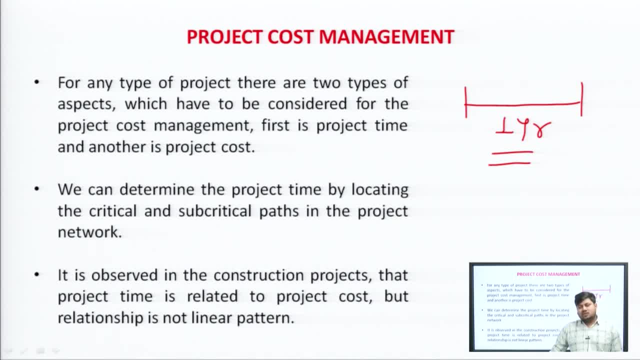 activities in our project. Why will we see the subcriticals and critical activities? will see that these are the activities that help to reduce or increase the project duration. If there is a critical activity, then we cannot reduce it in it. we can reduce it in the subcritical. 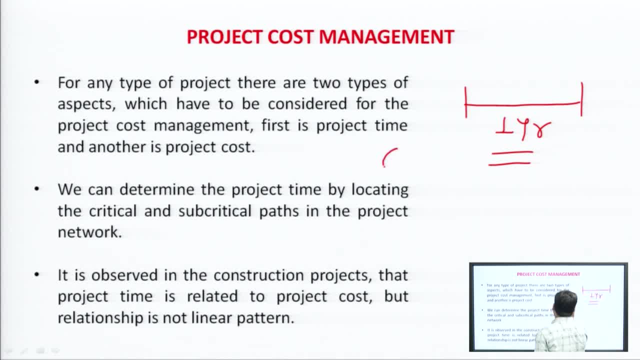 So any activities, which activities, critical and subcritical activities- we will have to see these activities which will basically be dependent on reducing our project cost or to make it optimum. Now we have seen one thing: that, as in some projects, the project cost is increased. the 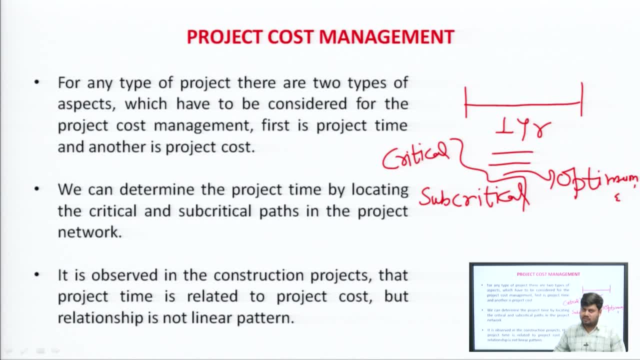 project time is increased, so along with that, the project cost is also increased. In some projects the project time is increased, so the project cost is also increased generally, But this is not linear. in relation to the pen, This means This means that there are some extra costs. between these two there are some different. 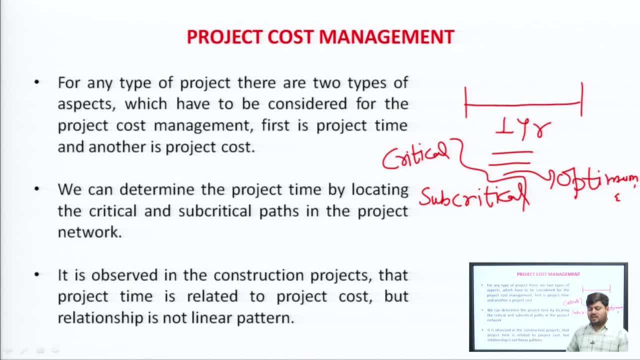 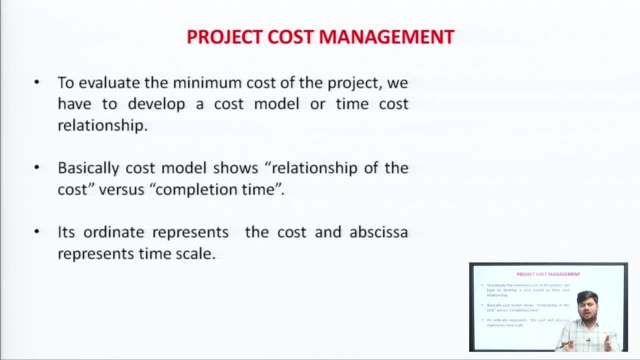 types of costs that basically affect them. So, in a simple way, we have to manage this project cost in such a way that our time as well as cost can be evaluated simultaneously. To evaluate the minimum cost of the project, we have to develop a cost model. 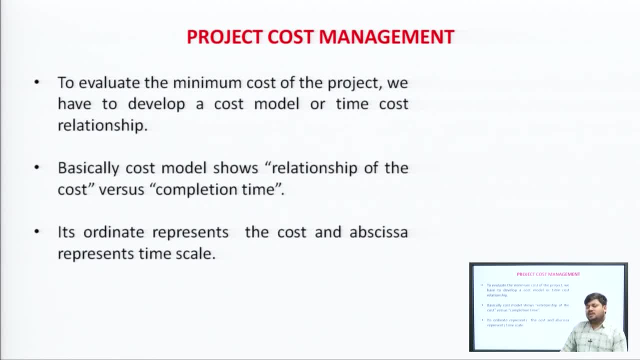 Very good, We will have to make a cost model. What is a cost model? Cost model means we will have to make a graph in which we will do analysis that the cost is varying with our time. In what way are they varying? Why are they varying? with which activity? 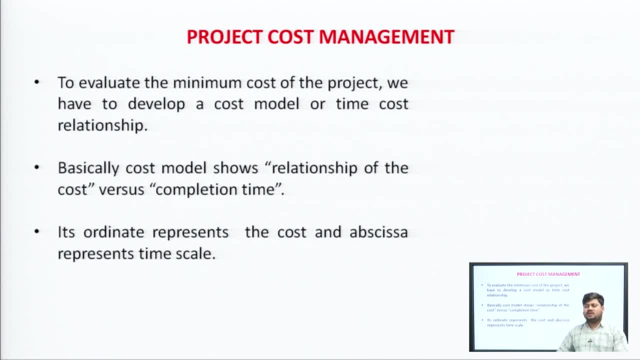 So we will find out the activities in which we can reduce our time. we will see them. Okay, Basically, the cost model shows the relationship between the cost and the completion time. Okay, And its ordinate represents the cost and the time scale. 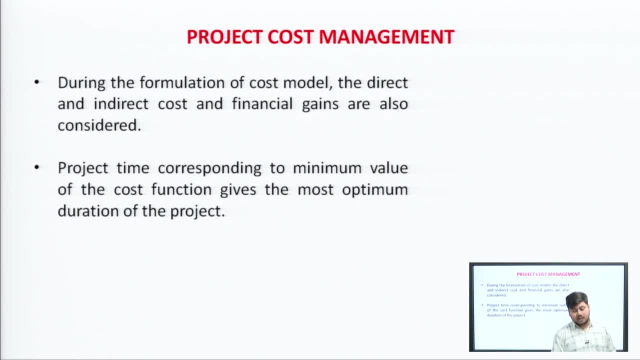 Okay, During the formulation of cost model, the direct and indirect cost and the financial gain is also considered. If we make a cost model, a cost model will basically be a curve in which a graph will be drawn. In the curve that is formed after the graph, we mark the optimum time and optimum cost. 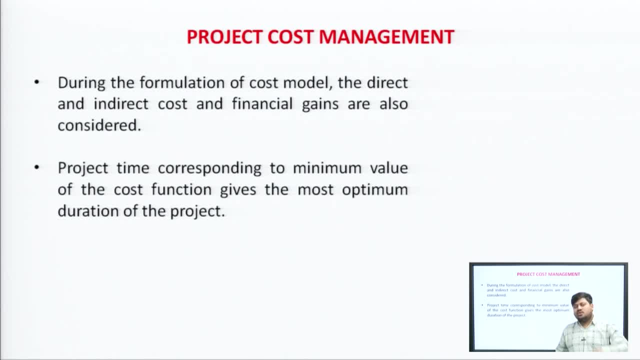 analyze the optimum time and optimum cost and try to bring the same time in our project cost. We try to bring the same cost in our project. This is called cost model. Project time corresponding to, basically, minimum value of the minimum value of the cost function. 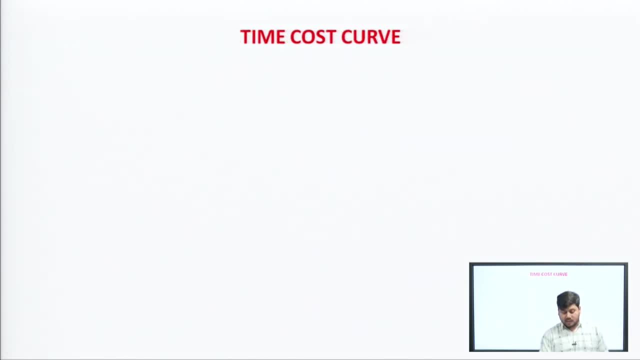 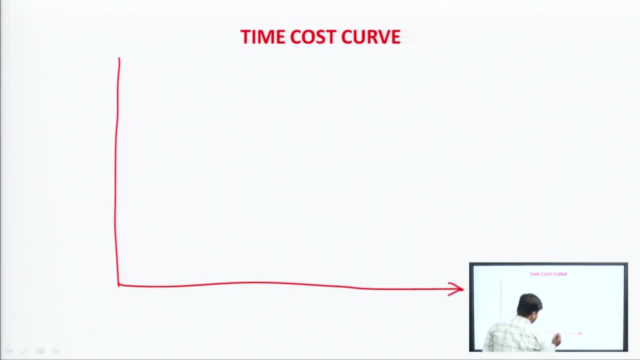 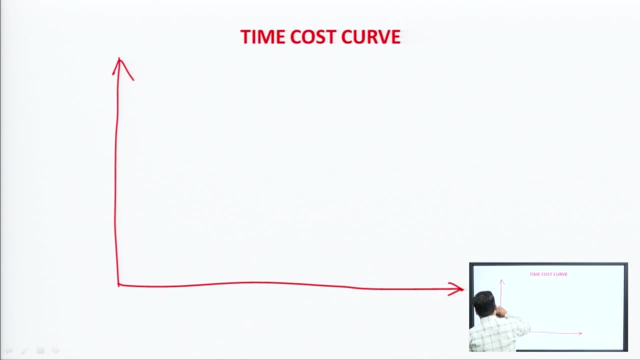 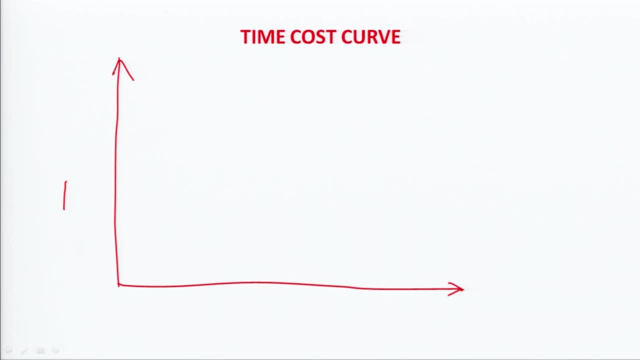 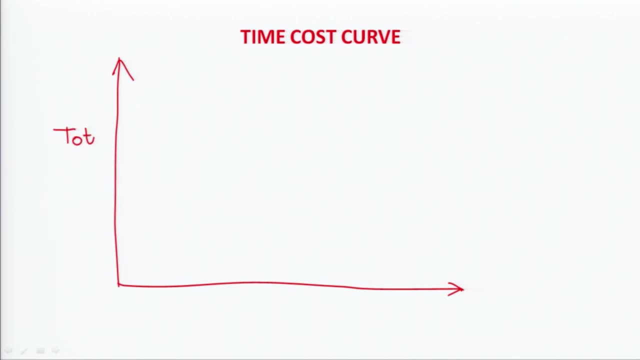 So if we draw a time, cost curve will be taken here total cost- and the excess will be taken here time duration. Now the curve is made in this way in which cost- direct cost and indirect cost- are all valid. 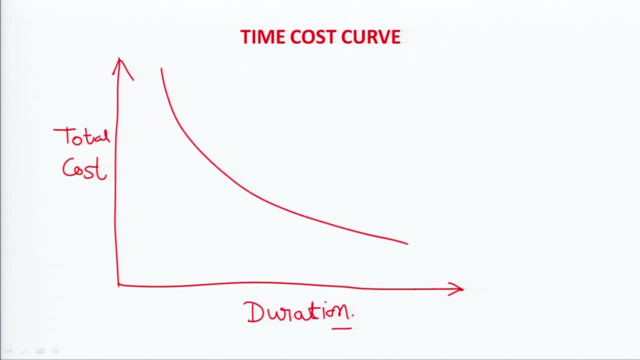 Now what is direct cost and what is indirect cost? we will understand after this. So this is the time cost curve. this curve is being made. this is the time cost curve. time cost curve. according to this, this curve is made in this way. this curve is made in this way. 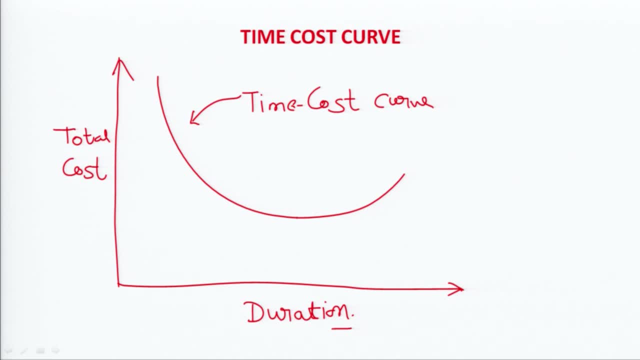 ok, So the minimum point that comes in this curve, we will calculate that minimum point, So the minimum point where we will cut from the x axis and from Y axis, then the minimum point where we will cut from the Y axis, which is minimum point, which is cut from the total. 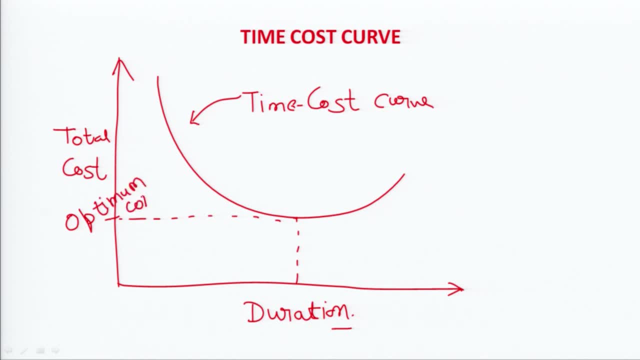 cost. We call it as the optimum cost or minimum cost. This is also called minimum cost. We try to bring minimum or optimum cost for our project And the cut which comes with this and the cut on x axis. we can see this in this principle. 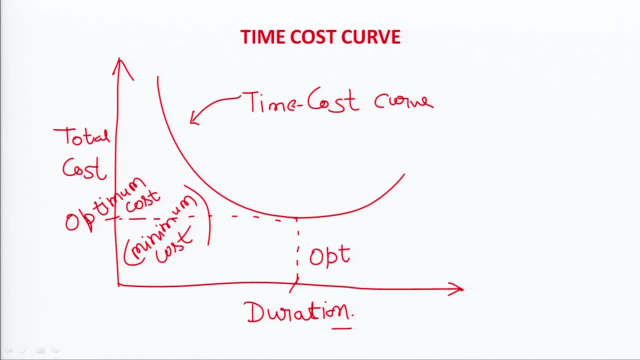 So we call it optimum duration or minimum time. optimum duration or minimum time or duration. So this is the curve in which the direct and indirect. what are the things in it? what are the things in it? there is a direct cost in it, there is a direct cost in it. the curve, 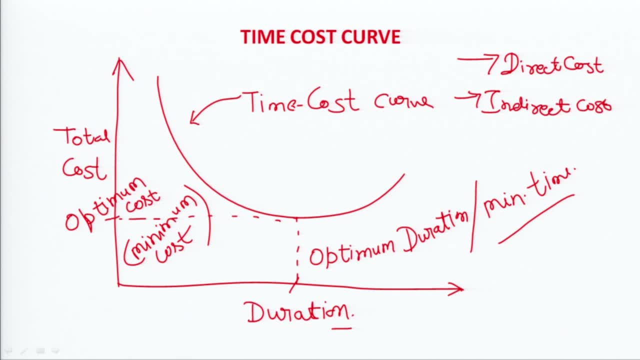 that is made of all these is called the time cost curve. From the analysis of this curve, from the analysis of this curve, we do time cost management in any project. basically, we do cost management and bring the cost of our project to the optimum. 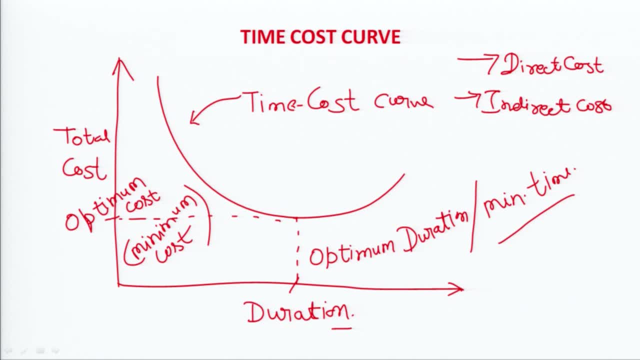 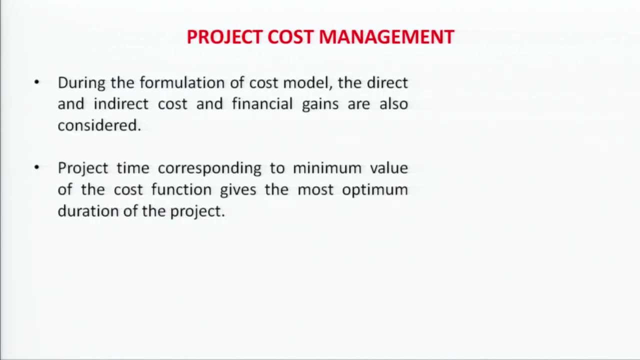 cost. We have tried to bring the time of the project to the optimum time. So this is the curve. This is a. this is a simple time cost curve. So some terms which is related to this, this time cost curve, we will understand. 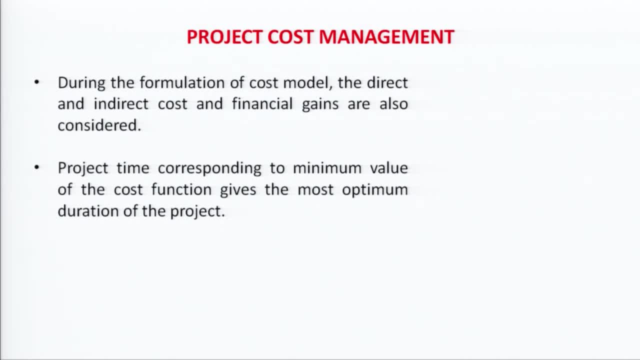 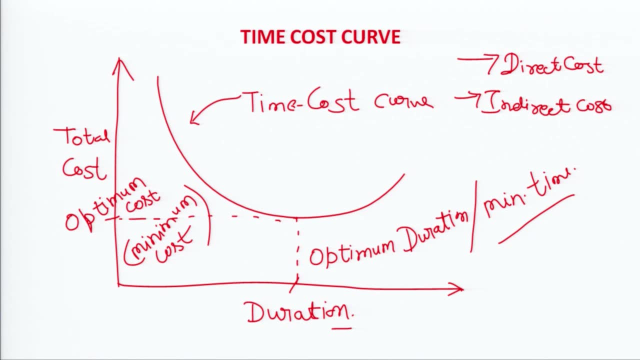 So the project time corresponding to the minimum value of the cost we have seen In the project curve, in this time cost curve. the minimum time is coming, the minimum point is coming, So the cost that comes to it, the optimum cost that comes to it, the corresponding time. 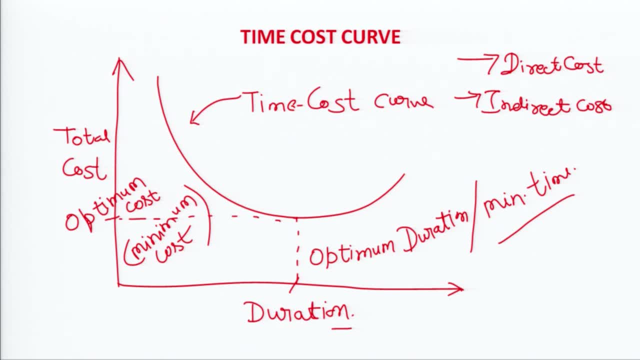 comes from it. It means it takes as much time as the cost, For example. let us take three examples. Like the previous one, we have two, three types of projects, three contractors who are doing the project. How One contractor is saying that we can do the work in 10 lakhs. 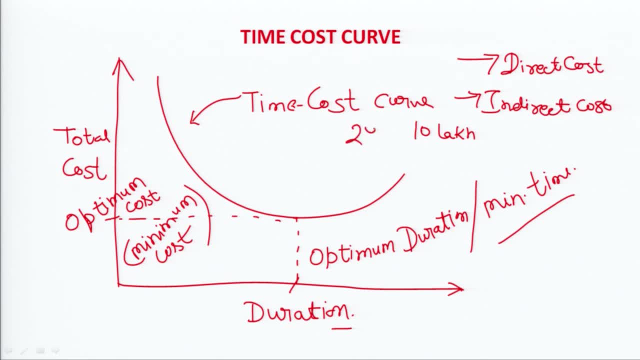 Ok, But the time it will take will take two years. One is saying that we can do it in 15 lakhs, But the time it will take is one and half Means one year and six months will take, But one is saying that we can do it in 20 lakhs. 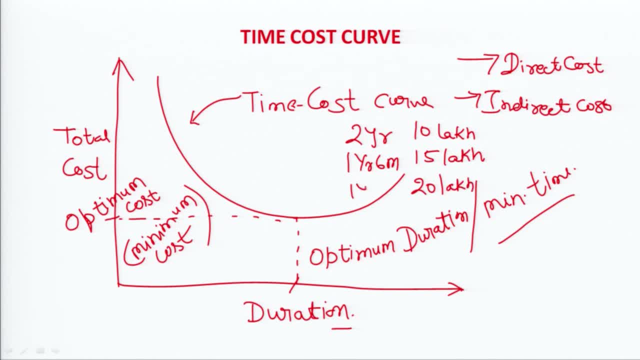 But the time it will take. for example, it will take one year. So if we talk about all three, then in the first one the cost is very less, less than the optimum cost, But the year time is very high. 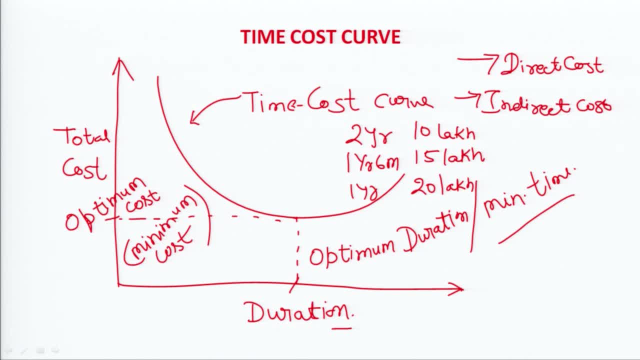 In the second one the cost is medium, Ok, And the time is also medium. And in the third one the time is less but the cost is very high. So we will have to choose one of the three, which is our optimum, which is right for us. 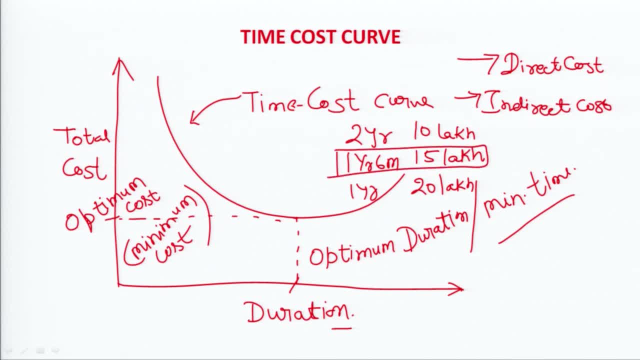 So we will choose the middle one. So we will call it the optimum cost: 15 lakhs And the corresponding time of the optimum cost. we will call it. it means what will be the time in which the optimum cost is taking place. we will call it the optimum cost. 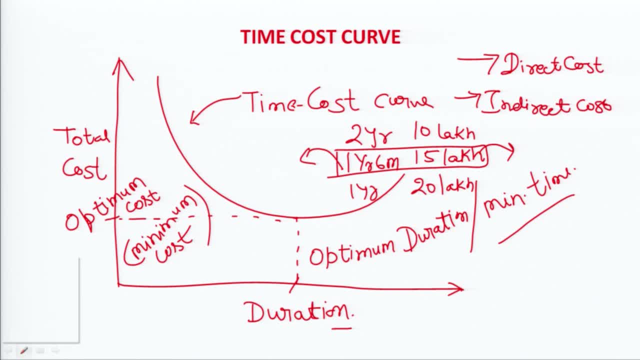 So the cost that comes in this way is called the optimum cost And the corresponding time of the optimum cost is called the optimum time. Ok, So we will remove it. We will see the curve, We will make the curve, Ok. 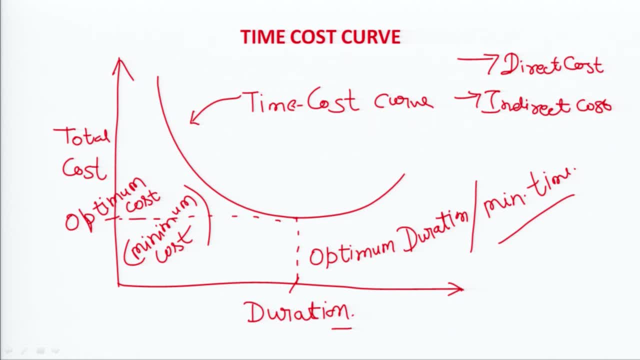 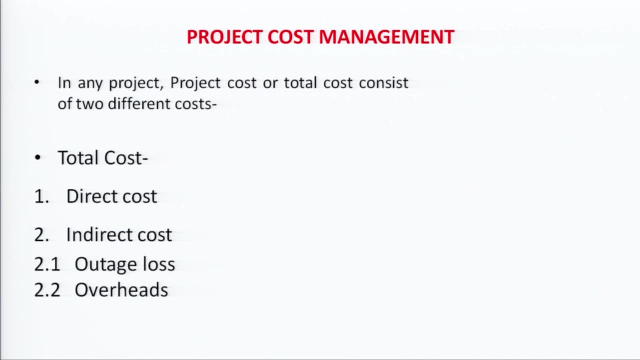 Now there are some terms like direct cost, indirect cost. We know about it, Ok. So before that, Ok, So for this, in any project, there is a total cost. Basically, there is a total cost. This is the total cost. 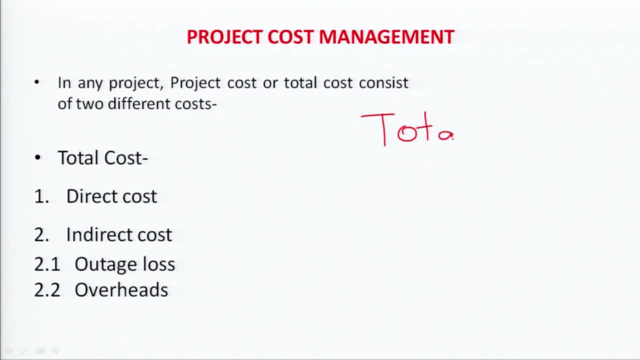 Let us try to make a diagram of it, A chart. There is a total cost. In that total cost, there are some different costs. For example, the total cost is made up of our direct cost, Direct cost, And the total cost is made up of our indirect cost. 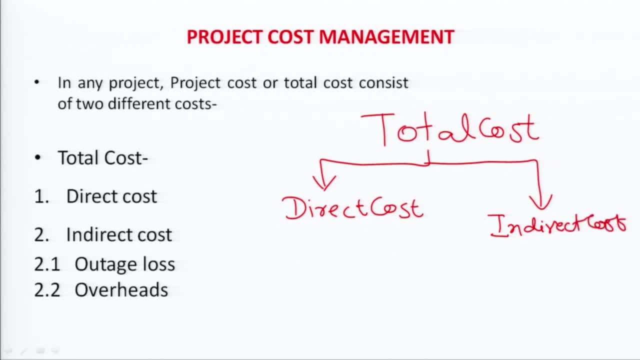 These indirect costs are made up of two types of costs. The first one is outage losses- Outage loss- And second one is overhead Overheads. Ok, These are the some costs which is related to the total cost. Ok, related to the total cost of the project. There are two types of cost which is related. 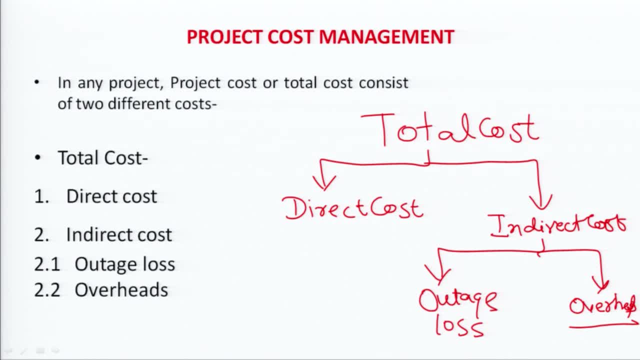 to the total cost. First one is direct cost. what is direct cost? we will understand. And the second one is indirect cost, which terms? which is we also subdivided into the outage losses and overhead courses. So what is a direct cost, We will understand direct cost. 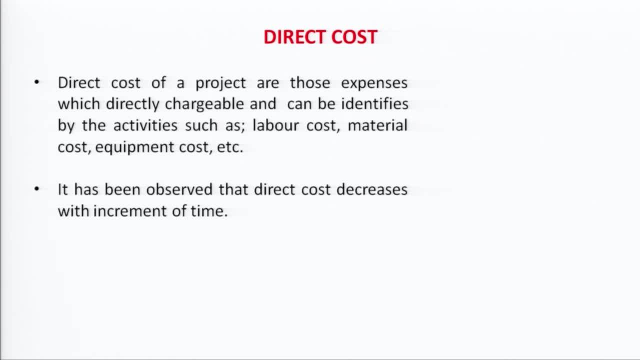 means the direct expenses. direct expenses which we have to pay, For example the direct cost which is directly charged. it is called direct cost. It is called labor cost, material cost, equipment cost. We know the cost which has to be paid, Which cost, The cost which. 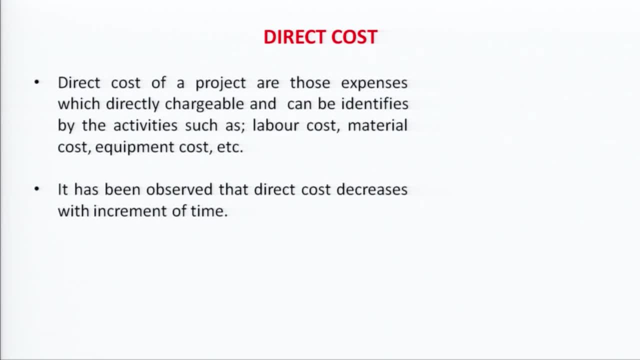 has to be paid directly, which is known for our construction, which is known initially. it is called direct cost. It is basically a cost. What is the cost? It is our labor cost. We have to pay the material cost and also the equipment cost. 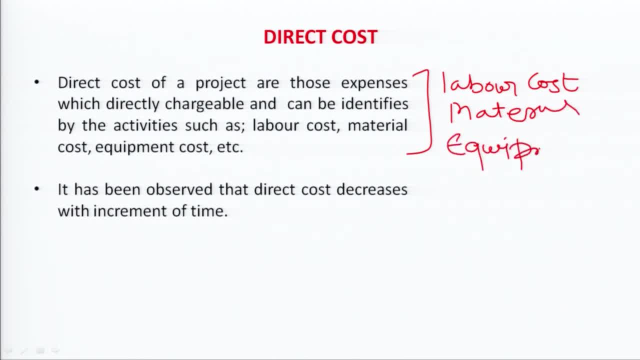 Ok, This direct cost, which is generally seen the direct cost. it decreases in the increment of time, Increasing the increment of time. the time increases. the direct cost decreases because material is to be paid initially. The material cost is basically the initial cost. 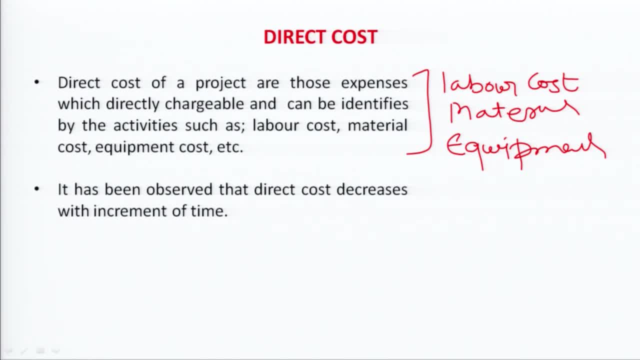 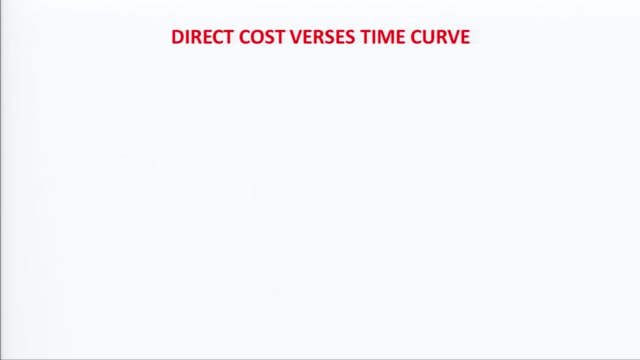 Ok, but in the case of dire cost, the only thing that we will discuss is it goes up with time, which is increasing, increasing, increasing. the more time is there, the more dire costs will continue to go up. If we look at the relation of dire cost with time, it keeps decreasing. 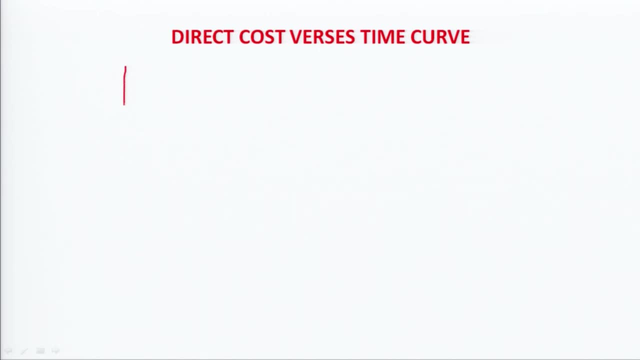 Basically, in the y axis we draw a direct cost and the x axis we generally draw a time, the duration, both of things. So the curve look like this: We can simple say that this is they say that duration, but as a time, but as a PCB time, PCB project curve this: 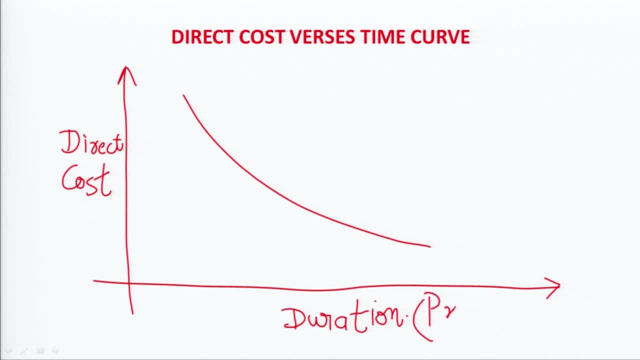 is a duration of which. what is duration? This is a project duration, project duration, project duration. So the duration is taking place, the duration is increasing, increasing and in the same way, our cost is being decreased, This minimum cost and any normal cost. let us assume that. 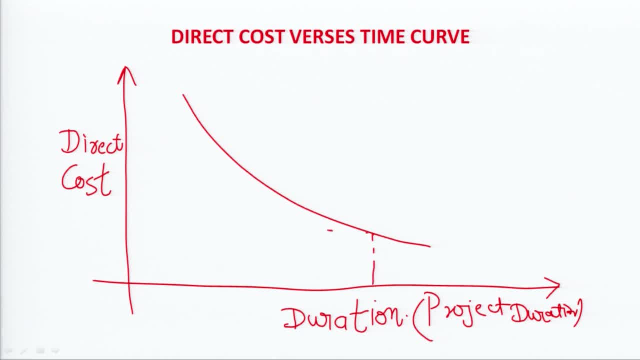 its a normal cost, so normal corresponding to normal cost. this is a normal cost, So this is a normal cost and this is a normal time. This is a normal cost, normal cost basically, and this is a normal duration and this is. 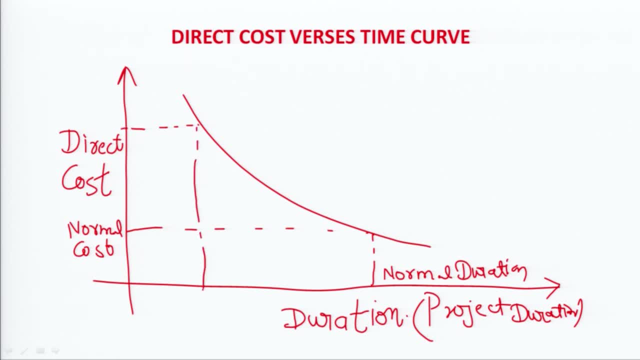 this point, treat as a crash cost. What is a crash cost? You will understand crash cost and corresponding the time, corresponding time to the crash cost, is a crash duration, a crash time, crash time, ok. What is this crash time? ok. 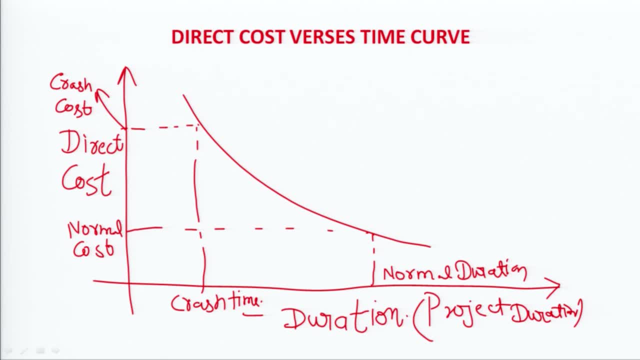 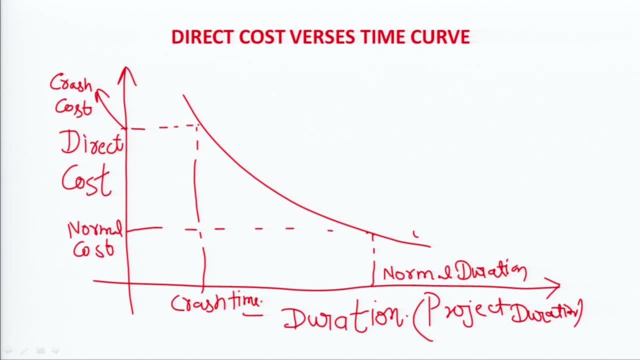 I aton time curve and this curve is called as a. this curve is a direct cost. the direct cost is versus time, how it is varying with time. simple, you can see it is carrying with time. 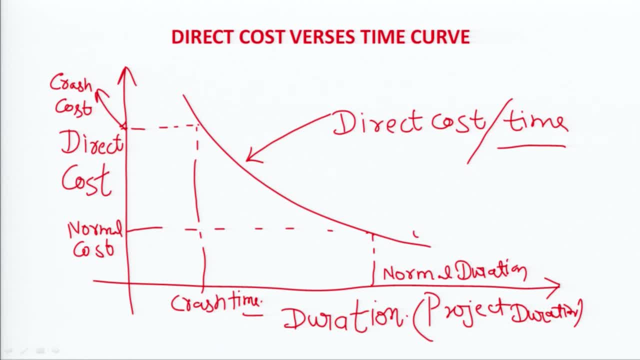 it is decreasing with time. direct cost will decrease with respect to time. in this way, a curve is formed which increases with time, which is called indirect cost. ok, So we have to write a balance of direct cost and indirect cost. at which point it is cutting? 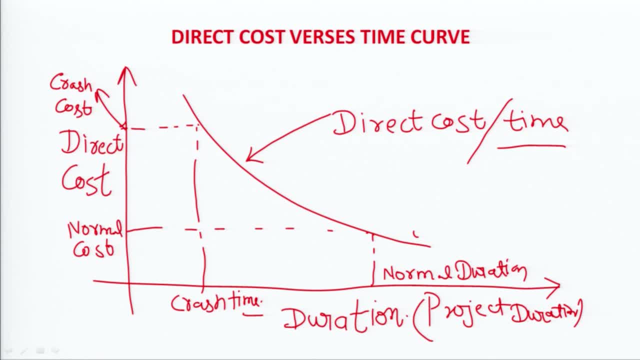 at which point it is balancing at that point, what value is coming at that point, what cost is coming at that point, what time is coming. by managing that time and cost, we optimize the cost of our project. We will see about this in the upcoming classes. this is a curve of a direct cost versus direct 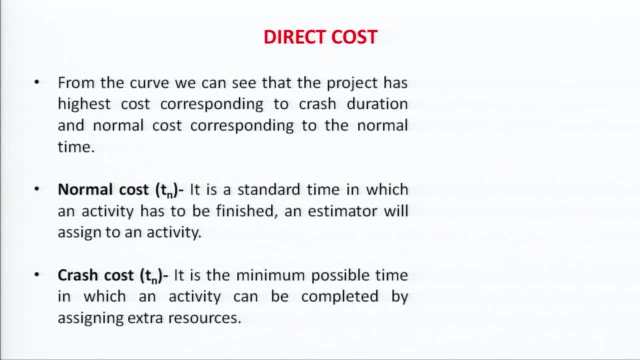 time curve, ok, So some term which is related to this curve we can see, So from the curve. So from the curve we can see the project has highest cost corresponding to the crash duration and the normal cost corresponding to the normal duration. we have seen it. 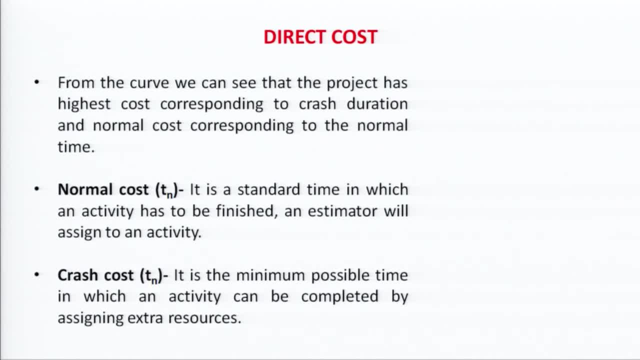 Now the normal cost and normal time, the crash cost and crash time. what is it? we will know about it. So first of all, first we understand the normal cost. normal cost is a standard time in which an activity has to be finished, a normal time. normal cost is such a time a. 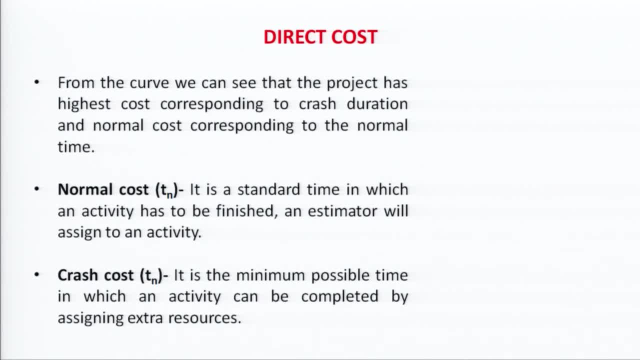 normal time on which our activity has to be finished. ok, who makes this? who estimates it? who makes this? estimator means the one who makes the estimation, who is taking the time and cost of any activity about that like an estimator. an estimator is doing some. 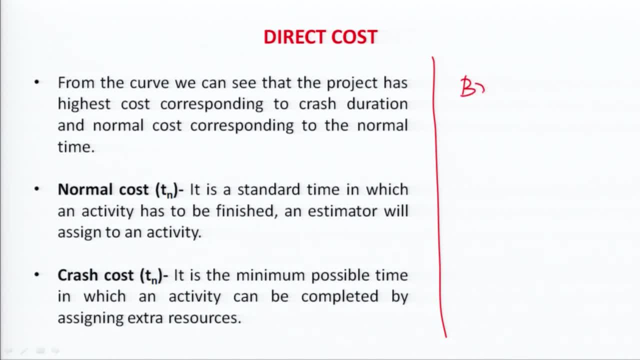 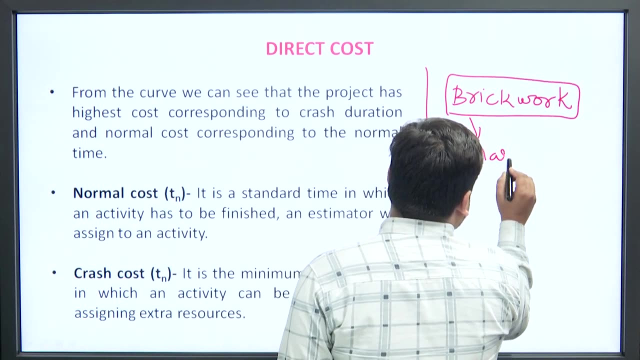 estimating. so he has done. a brick work means there was a brick work activity. brick work was an activity in which he assumed- he had to assume some assumptions- that in a particular wall two machines. Yes, Yes, 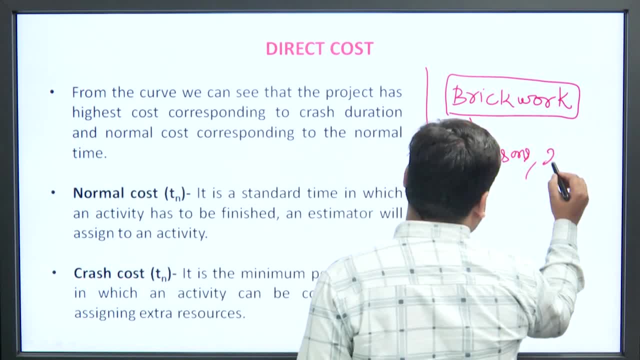 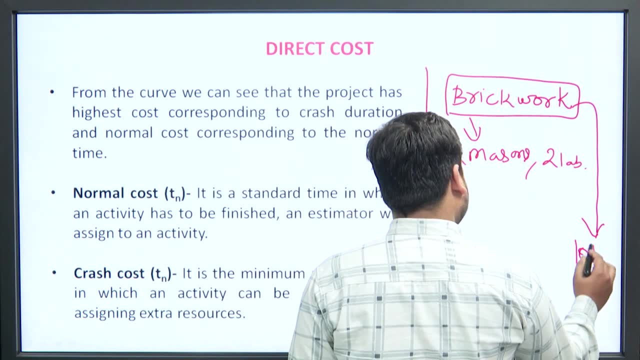 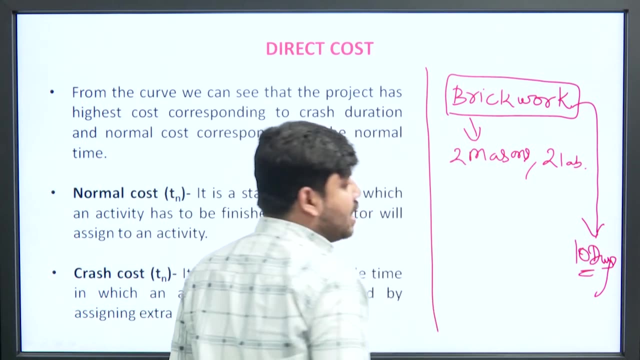 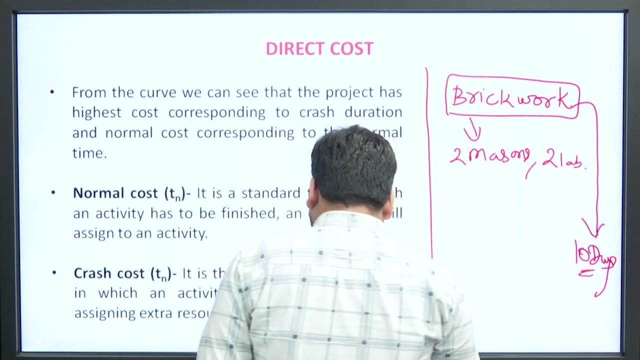 Yes, on this basis, it will take 10 days to work on this brickwork and some cost will be assumed. This 10 days will be called as normal time. duration of the activity and cost corresponding to this normal time is called as a normal cost. 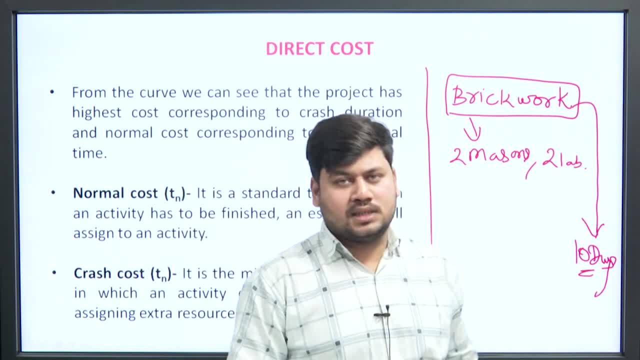 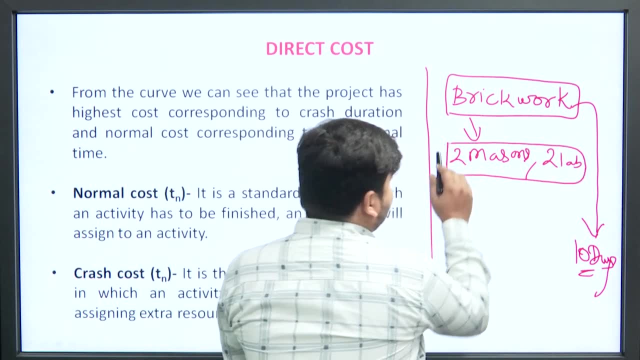 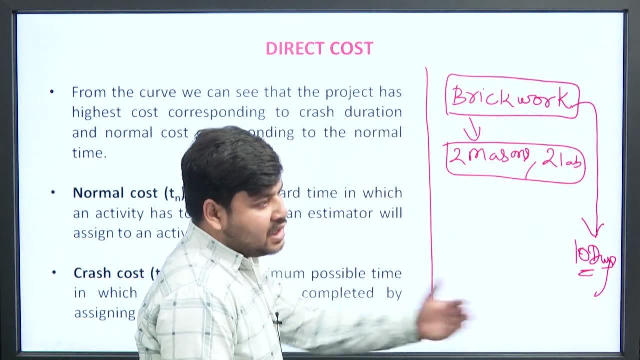 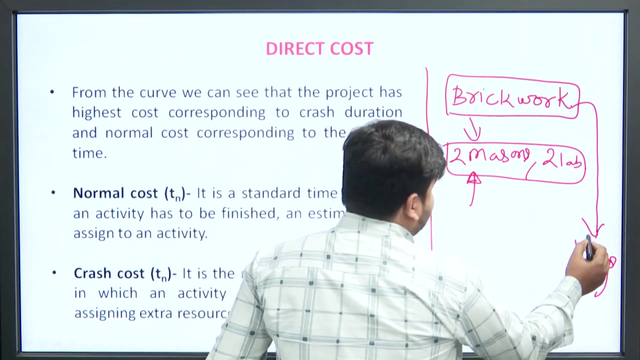 But if the work can be done in a short time, then we will have to increase the resources, for example the labor and the material. So if we feel that we can only do it in a short time, then we would need a lot of filling. 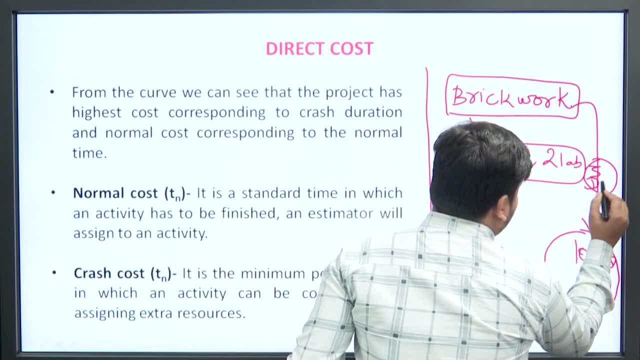 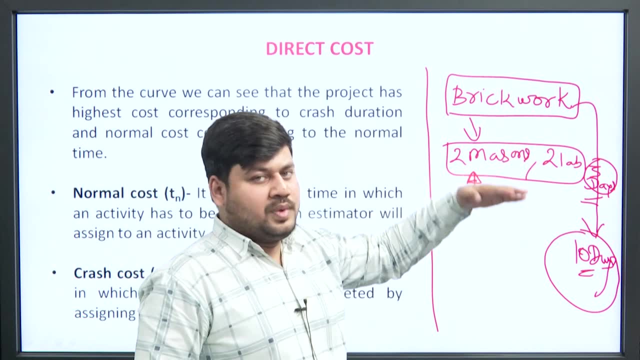 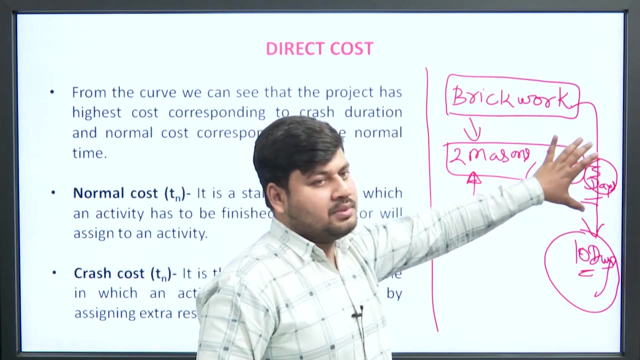 of investments, But we can't do it before 5 days. Why can't we do it before 5 days? Because the brickwork can't go above a particular height, Because it has to be set first, So we can limit it to a particular time. 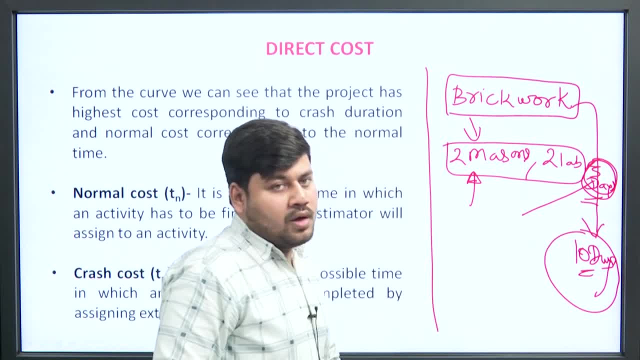 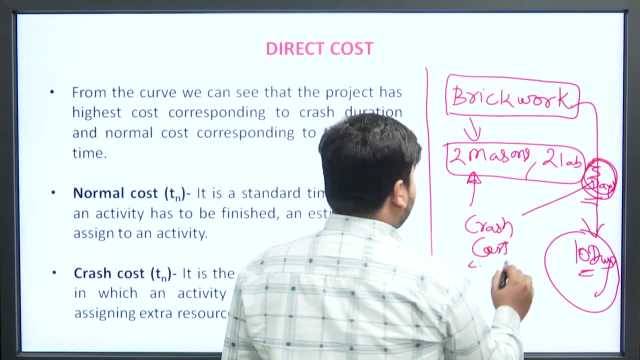 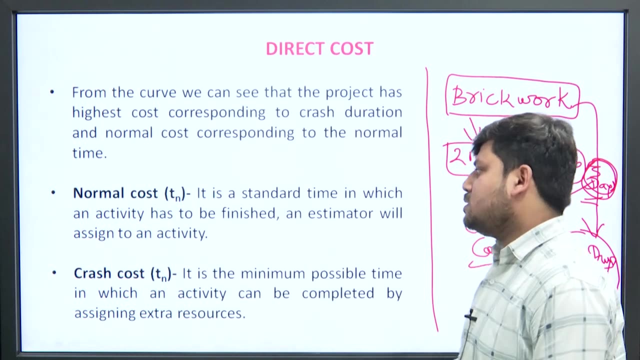 That particular time is called crash time. The corresponding cost of that particular time is called crash cost. So obviously, if we reduce something, then the cost will also increase. In simple terms, normal cost is a standard time in which the activity has to be finished And the estimator will assign a new activity. 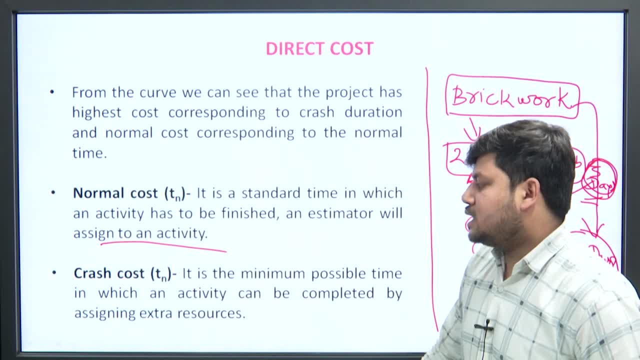 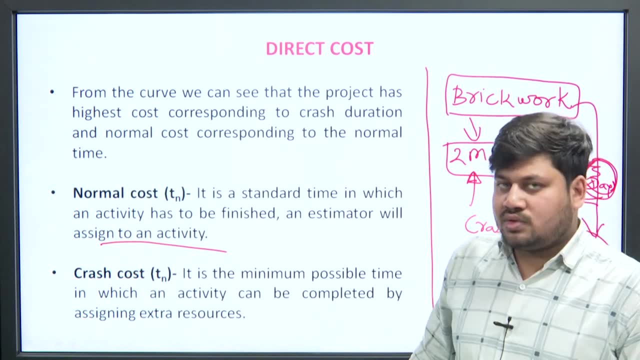 The estimator that assigns the activity has to be finished. Second one is a crash cost: Tn. It is a minimum possible time in which the activity can be completed by assigning extra resources. The minimum time is 5 days of brickwork In which we can add more resources. 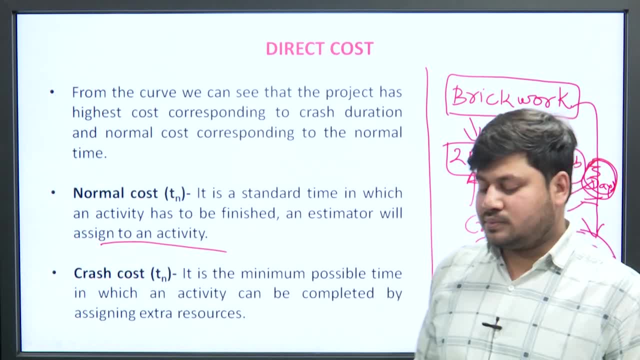 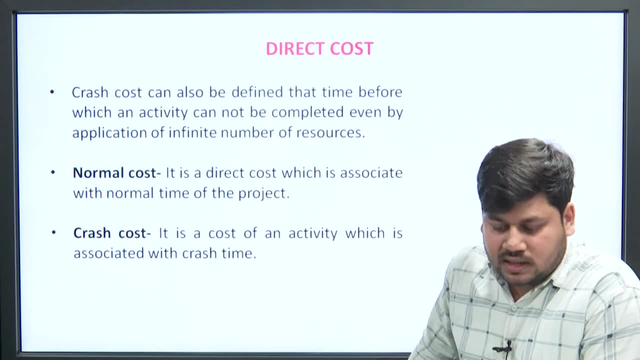 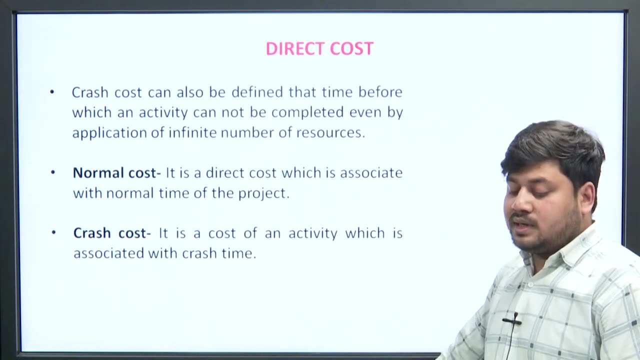 So we apply extra resources and make it work. So let's see some more terms. We can define crash cost in a different way. How can we define it? Crash cost can also be defined as the time before which an activity cannot be completed, Even the application of infinite number of resources. 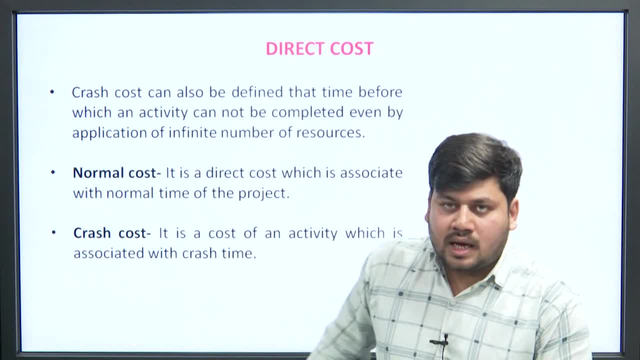 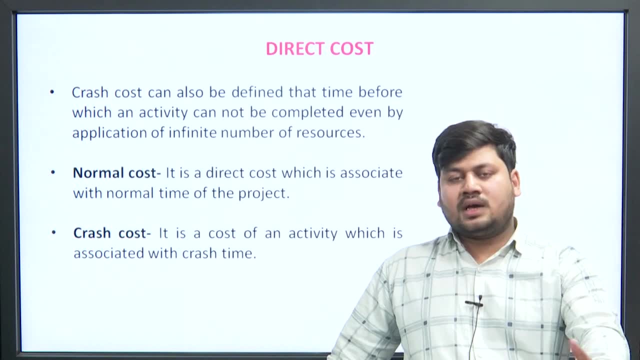 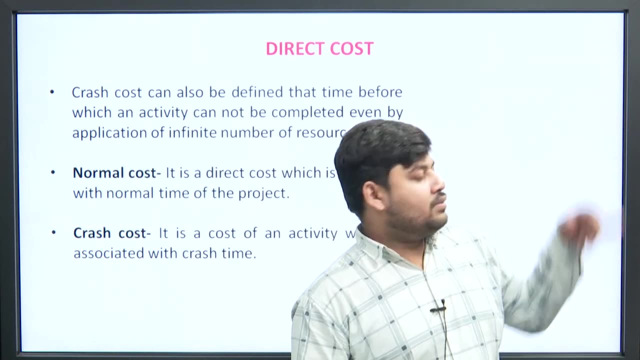 As we talked about setting it, Crash cost is that time. basically, That is the minimum time for any activity to be completed. If we want to go below this time, Then we can apply infinite resources, But we cannot go below that time. For example, if we make this brickwork, 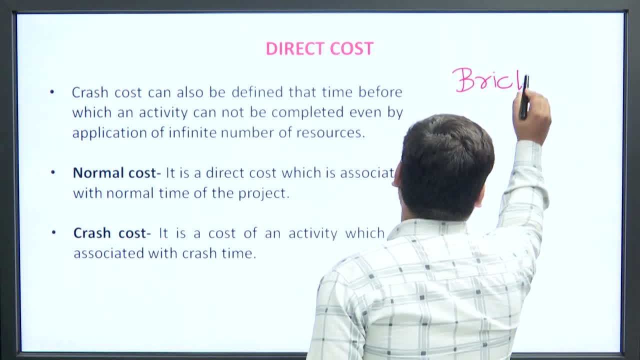 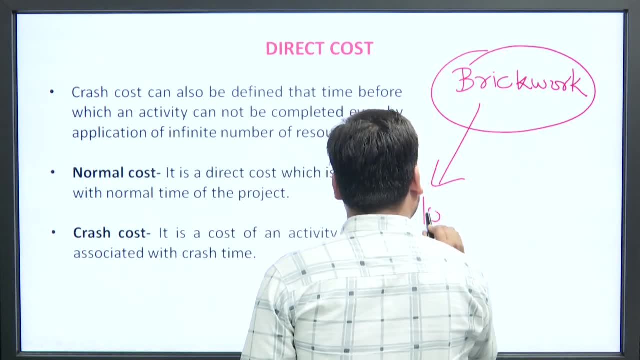 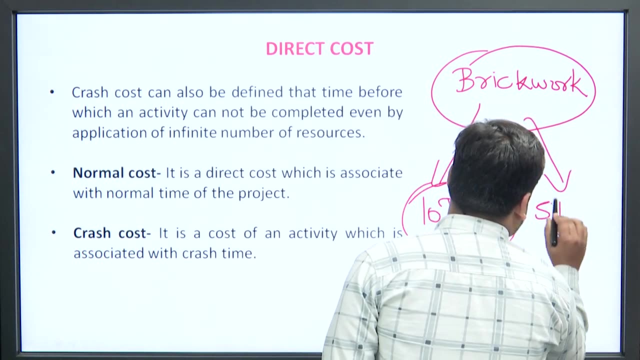 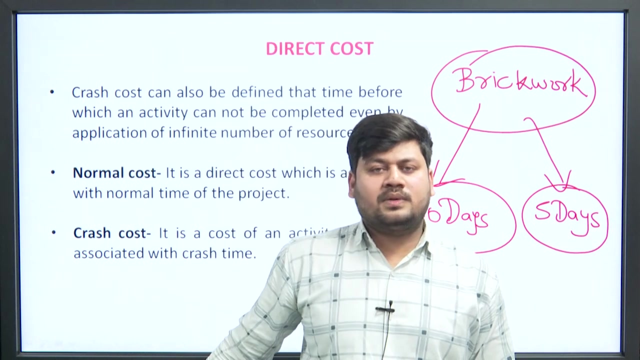 This is our brickwork. Brickwork's normal duration was 10 days And crash duration was 5 days, So we cannot do less than 5 days. Why can't we do? Because we have done brickwork. Why can't we do? We cannot go below 5 days. 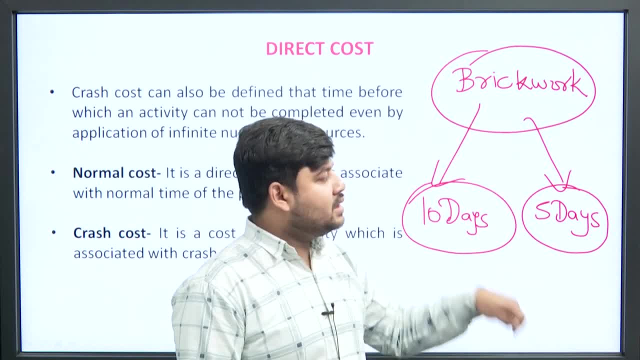 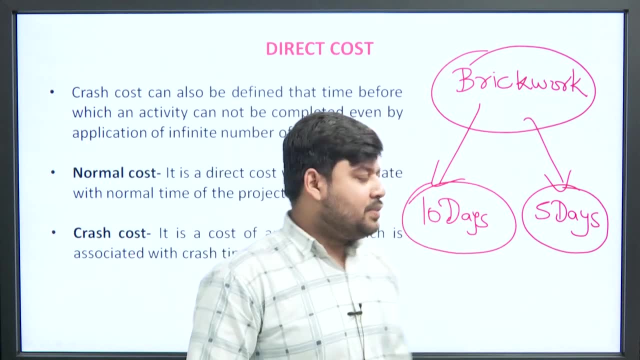 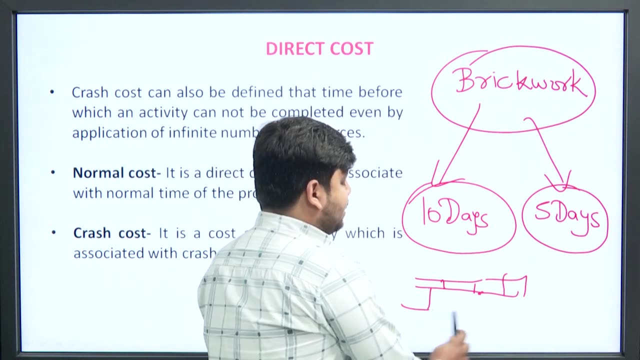 No matter how many resources we apply, How many machines we apply, How many labours we apply, But we cannot go below 5 days. Why can't we do? Because if we are doing brickwork, Then we have done brickwork till a particular height. Ok, So we can do brickwork above that time only. 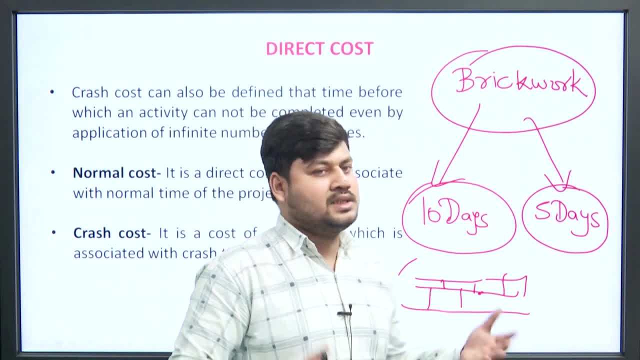 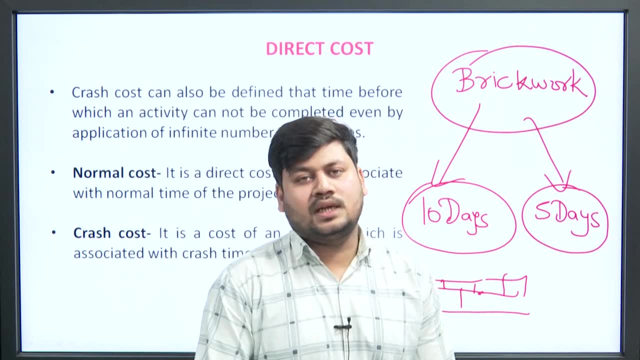 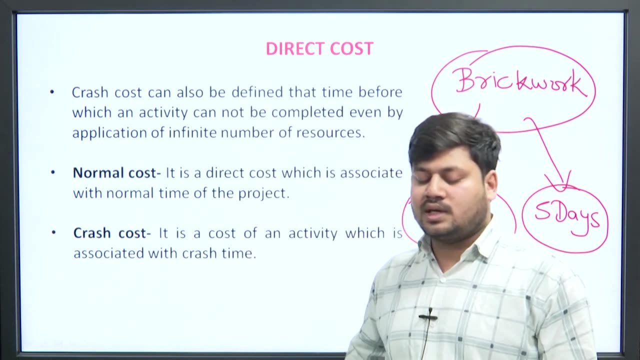 When the brickwork is set, When the motor is set. Otherwise, If we are doing brickwork above it, Then the chance of the ball collapsing is more So So. So it is a simple way. We have defined the crash duration differently. We have defined the crash cost differently. 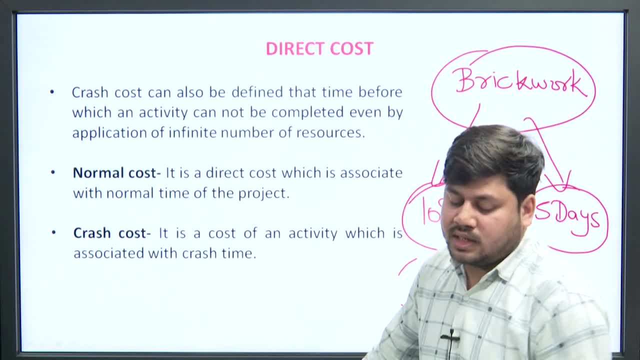 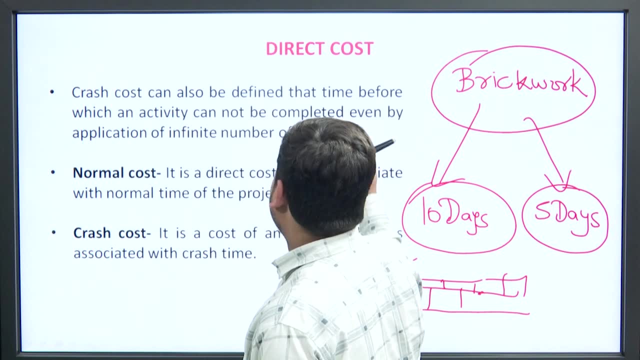 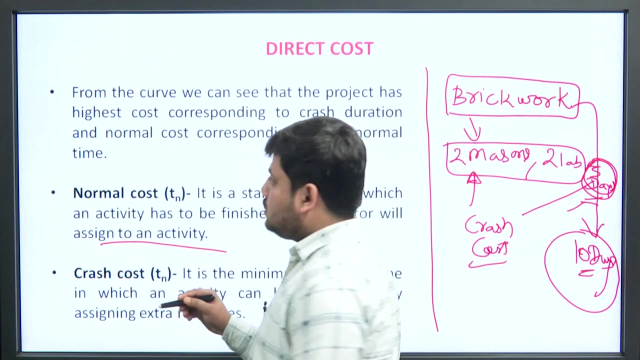 So crash cost can also be defined That the time, or crash time basically, Which an activity cannot be completed. Even the infinite Infinite, Basically this is a crash Time. Even the infinite number of resources: Basically this is a crash, Not a crash cost. This is a normal time And this is a normal. 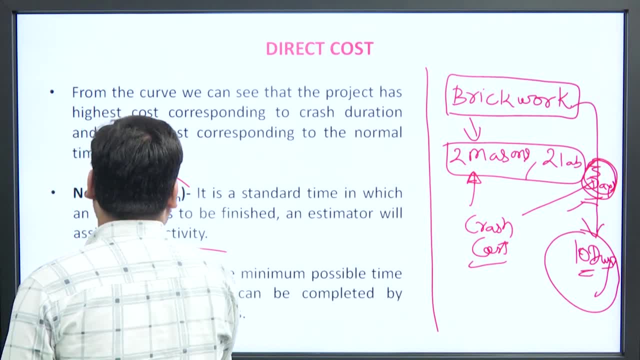 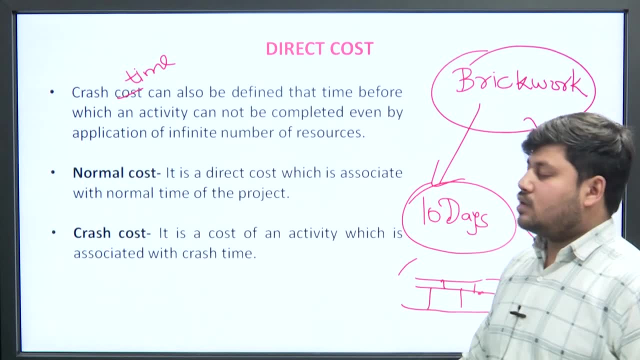 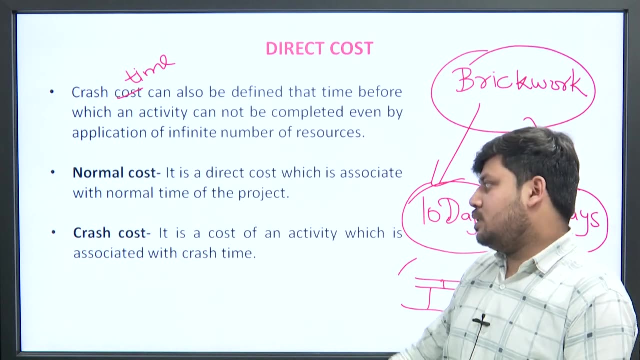 This is a crash cost. Sorry, This is crash time. Now we will understand about the normal cost And the normal Normal cost and the crash cost. Basically, The cost corresponding to your normal time is called as a normal cost. It is a direct cost which is associated with the normal time of the project. 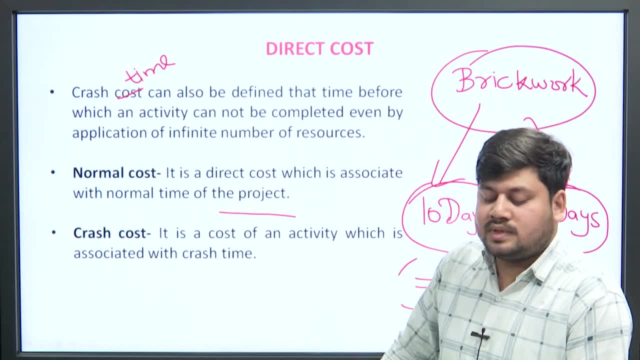 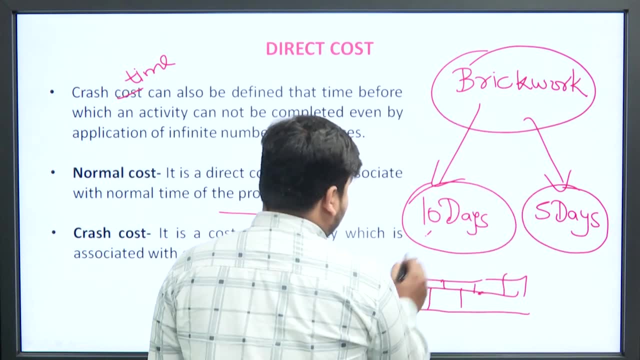 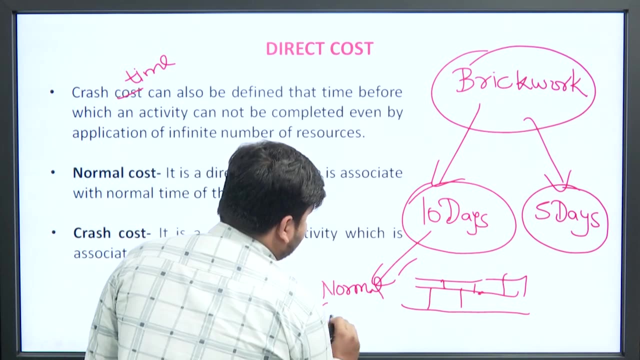 Also For crash cost is a cost which is associated with the crash time. Ok, The crash time is the cost. Basically, The money is being spent in 10 days. If we do this brickwork in 10 days, The money that is being spent is called as normal cost. 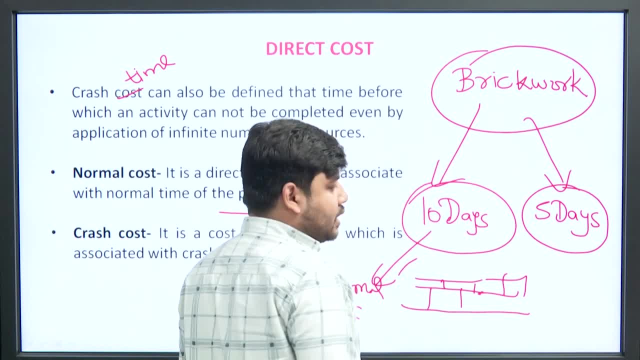 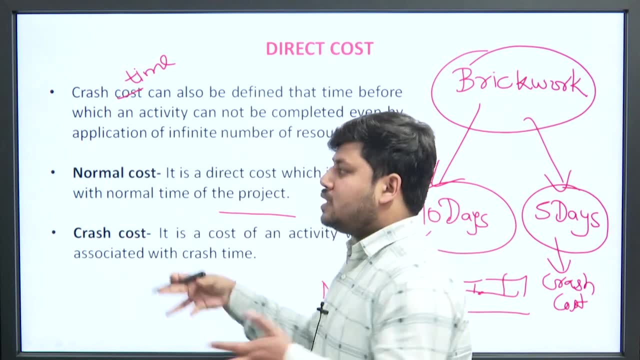 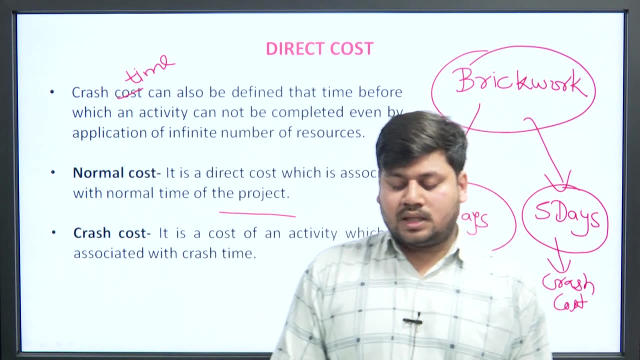 Normal cost And In 5 days, The minimum time that is being spent is called as crash cost. Obviously, The crash cost will be more. Why? Because We have applied a lot of resources together, So We have applied the resources together, So It will cost the resources, So The cost will be more. 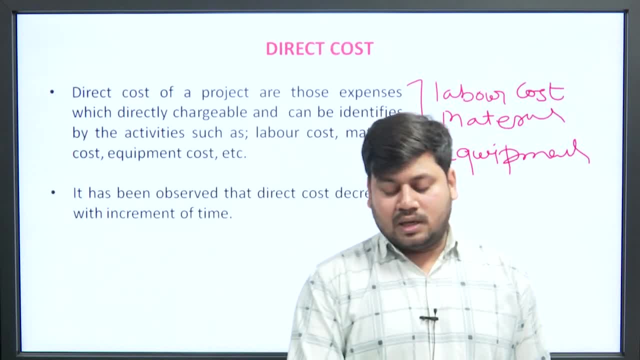 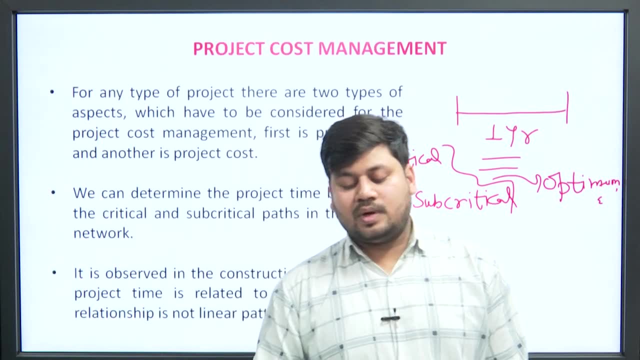 So This is all about today's class. We have seen a lot of things in it. We have seen a lot about direct cost And about project cost management, So We will do a brief summary of it once. So, First of all, We have seen project cost management. What is project cost management? 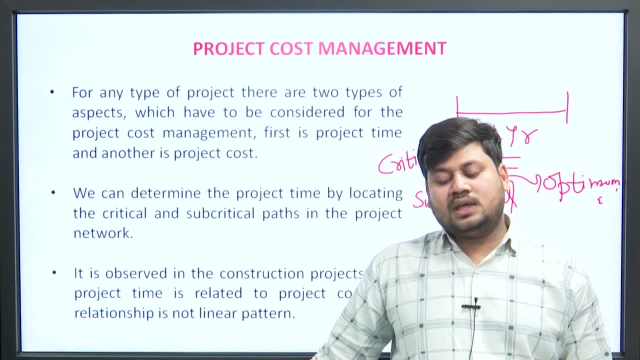 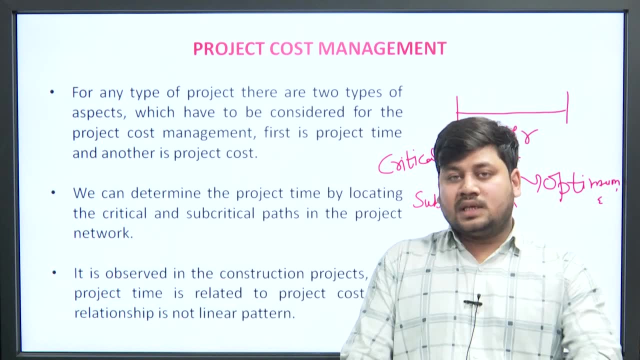 And What are the terms used in it? So, Project cost management: Basically, We have to manage the cost of our project. We have to minimize the cost. We have to optimize the cost. We have to minimize the cost By considering the project time also. Ok, We assume a time. 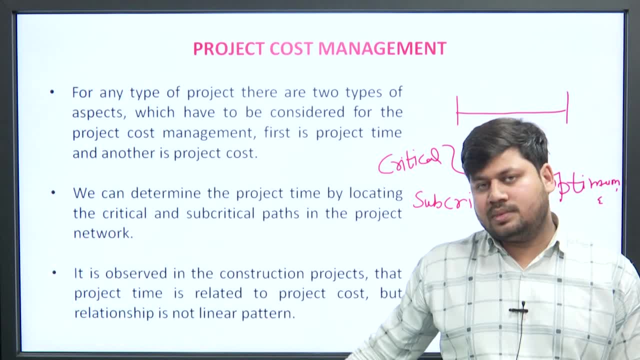 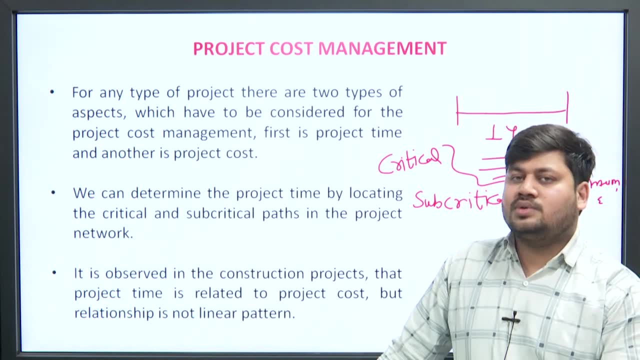 That Let's assume one year That the project is going to complete this activity. So In that one year We can reduce the activity of that project to a certain extent. That is called as project cost management. Ok, How do we do it? First, We Optimize our project. 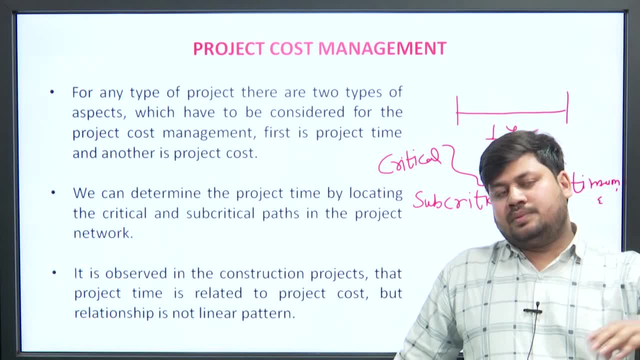 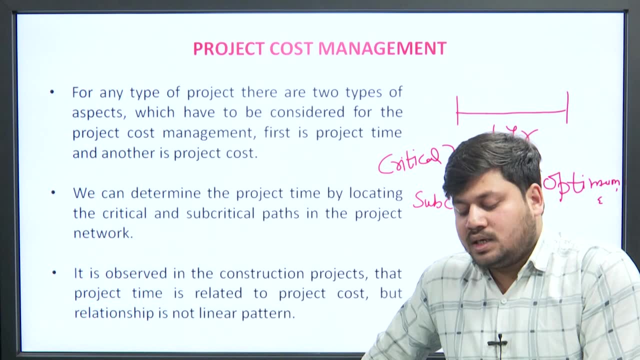 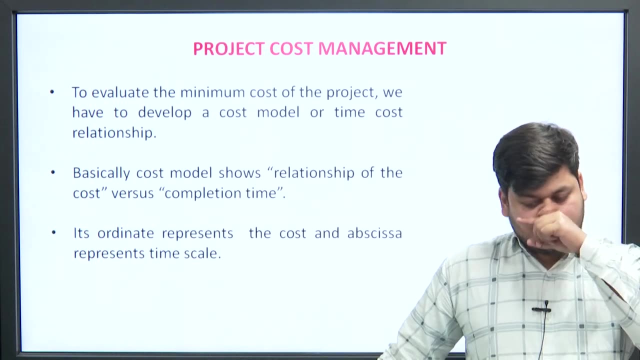 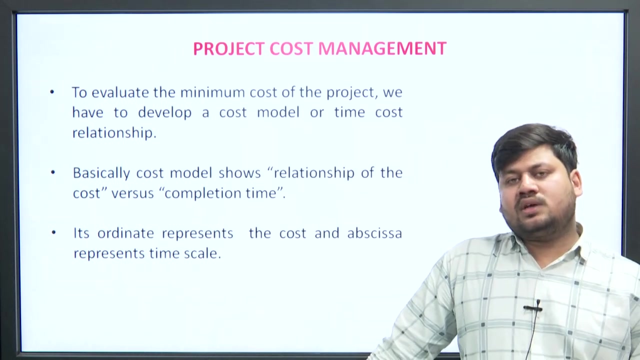 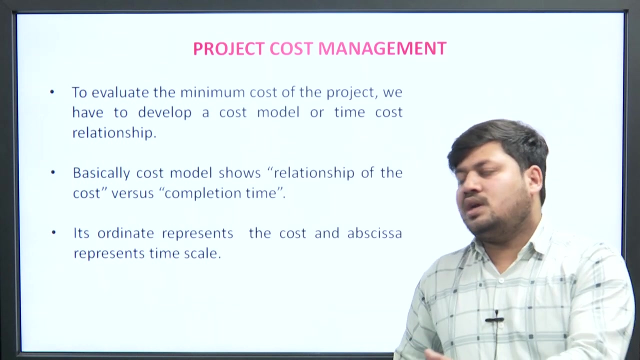 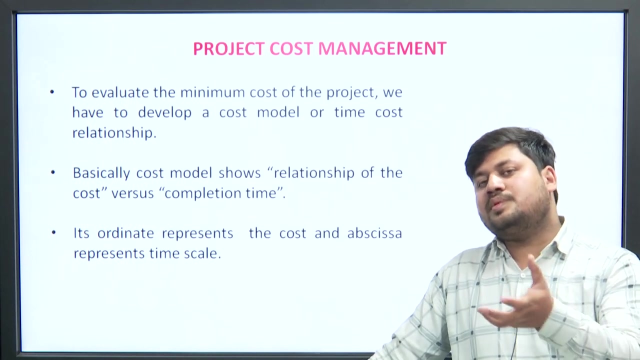 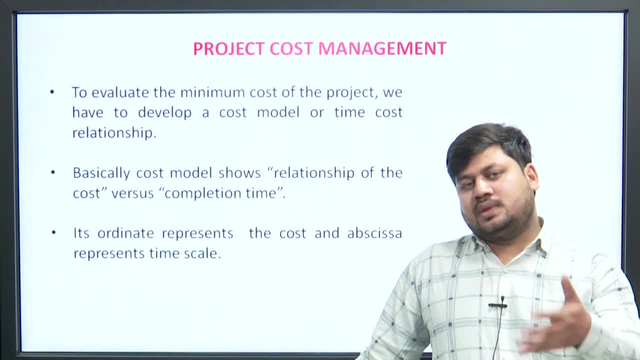 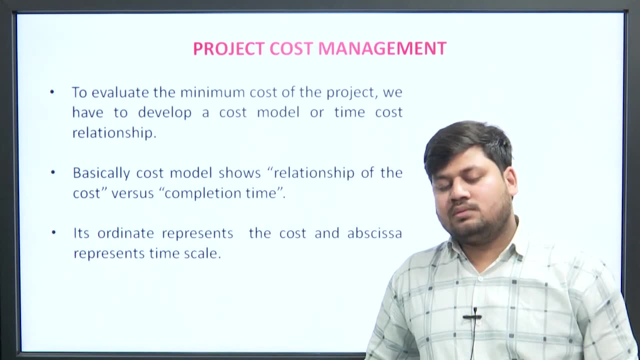 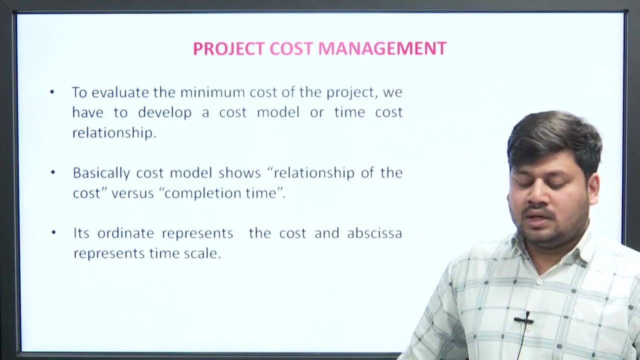 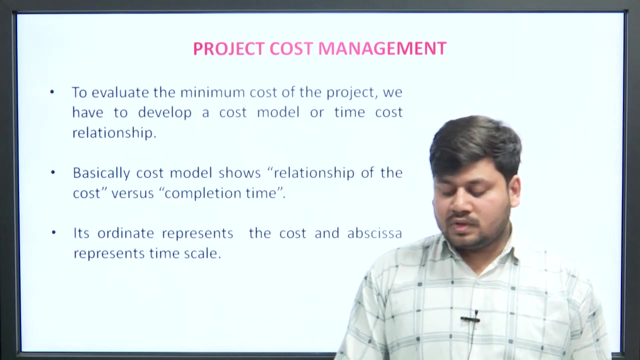 That is the cost that is being applied at that time can be the minimum. The corresponding time can also be the minimum. So we call it the optimum time and optimum cost. We find it and try it in our project. So basically, this post model is a relationship between our cost and completion time. 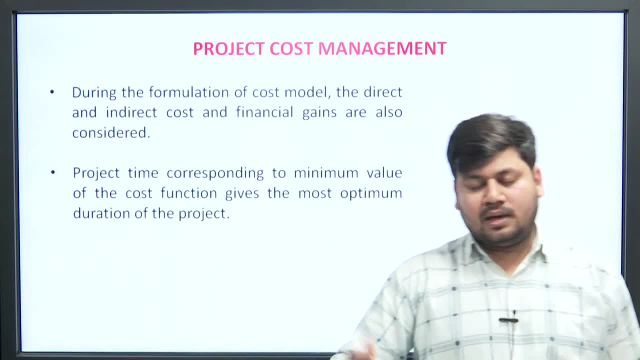 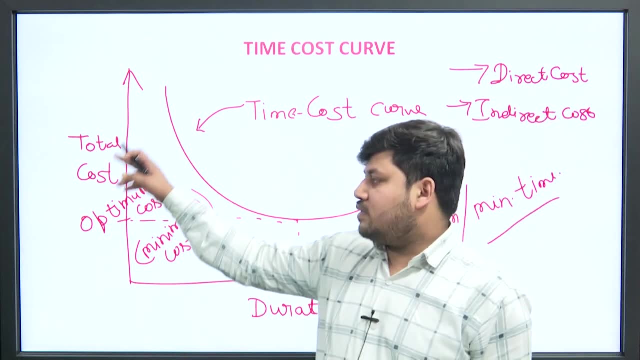 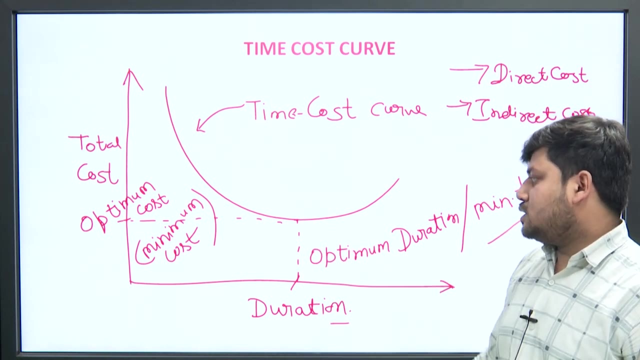 In which our ordinate cost depends on the time of the obstacle. We will also see. So we will see. This is a simple time cost curve in which the y axis is the total cost and the x axis is the duration. This is a curve at which a point which generates the optimum duration and corresponding to the optimum duration is called the optimum time. 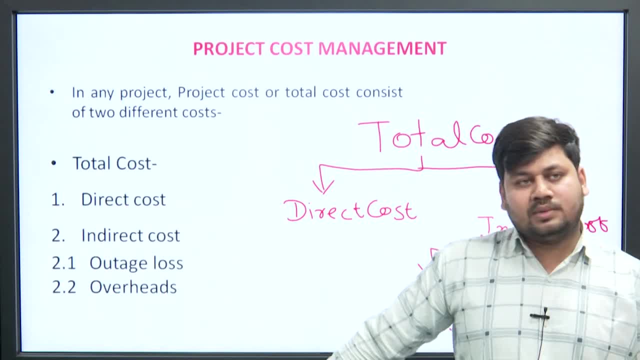 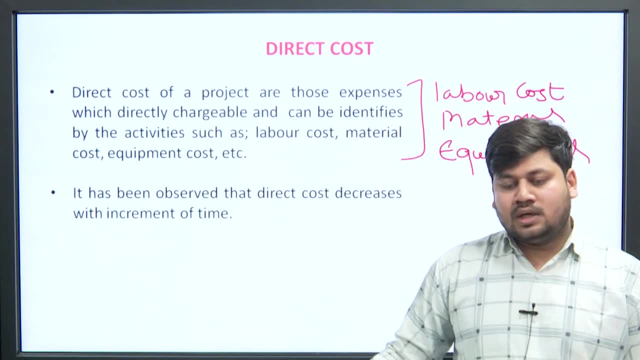 We try to find this. Then we saw the type of cost in project cost management Type of cost. we saw about the direct cost and indirect cost. Then we saw about the direct cost. What are the direct costs? Direct cost: we have labour cost, material equipment cost. all these are direct costs. 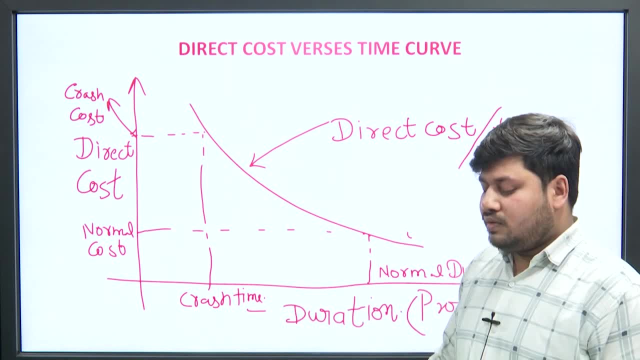 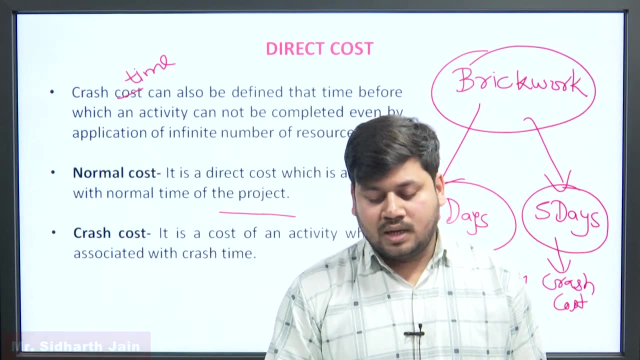 And in this we made a curve of direct cost Curve and in this we know about the normal cost and the crash cost. Okay, So this is the definition of crash time and normal time. This is the definition of normal cost and crash cost. Okay, So this is all about today's class. Thank you for watching this lecture.